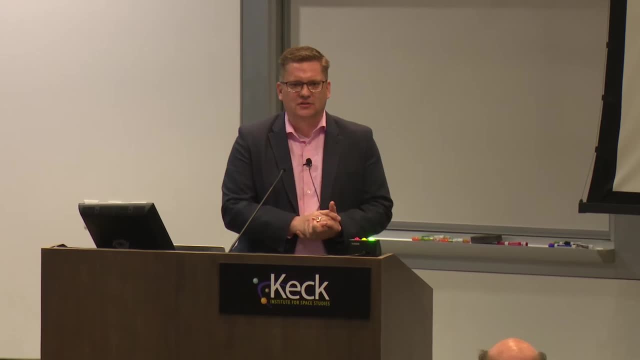 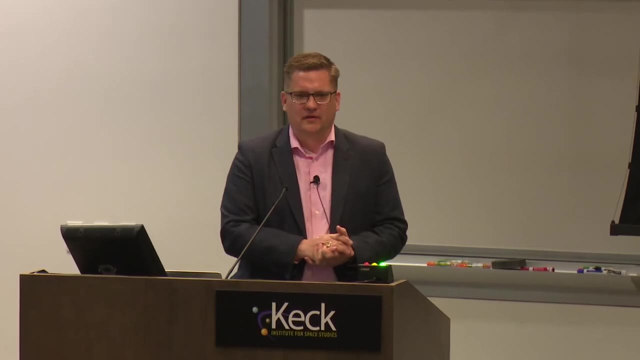 planets that I want to leave you with. This is a challenge to limit it just to five, because of course, our whole conference is devoted just to exoplanets, But I wanted to distill it down to the essential items that are motivations for this whole workshop. Many of these points, 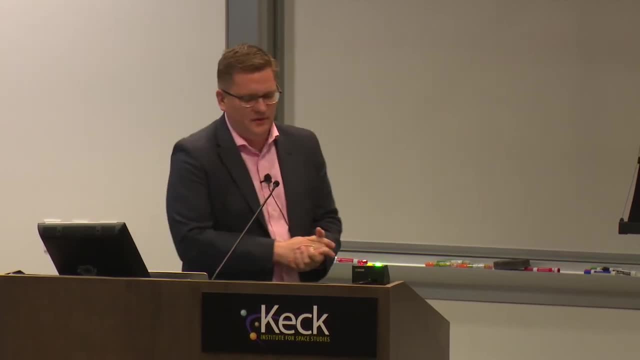 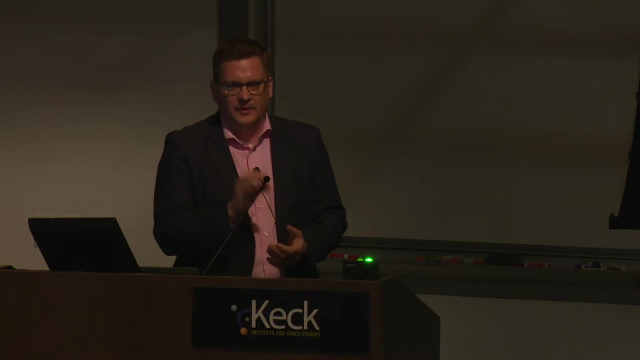 you've probably heard in the popular literature, but I want to emphasize them nevertheless. The first is that extrasolar planets are ubiquitous, And I want to be a little bit more precise about what I mean by ubiquitous. So most of our good demographic studies of extrasolar 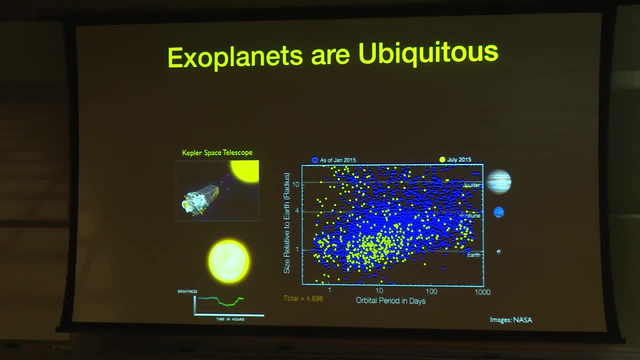 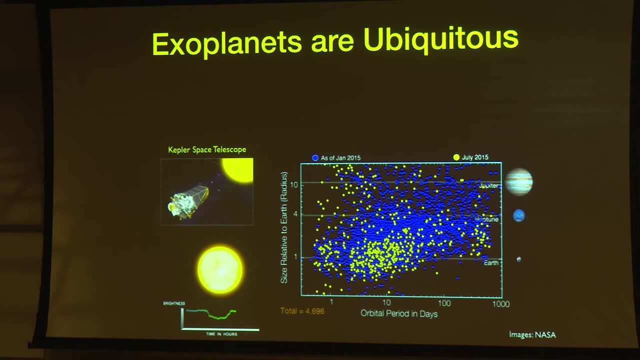 planets come from. the Kepler Space Telescope, launched a decade ago, ran for four years in its primary mission looking at a single patch of sky, where it conducted a census of 150,000 stars and discovered thousands of planets orbiting those stars using the transit. 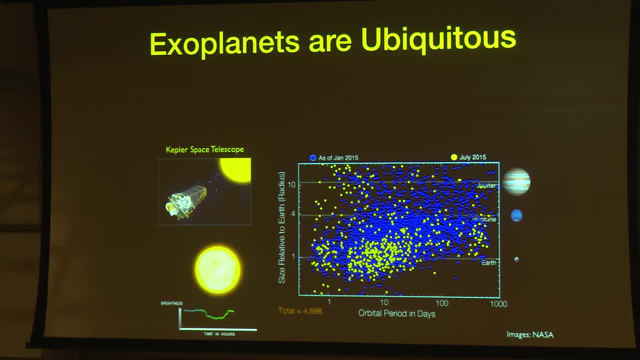 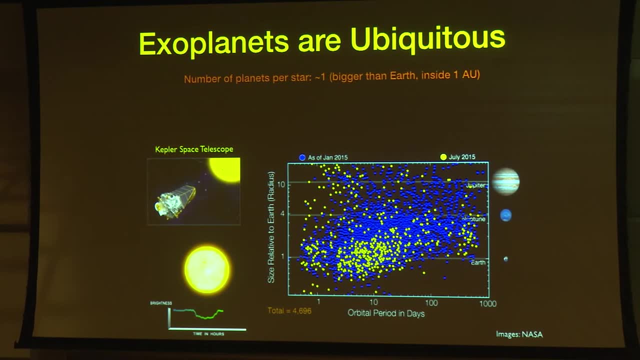 technique. One of the most important things about extrasolar planets is that they are ubiquitous, And one of the results of this census is that we now know that the mean number of planets per star inside of 1 AU and bigger than Earth is about one. That's a remarkable 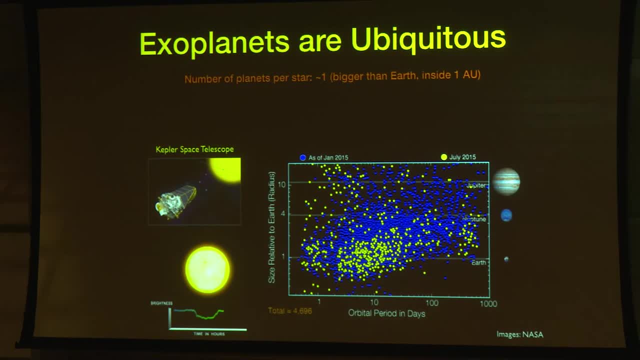 statement about the universe that the universe appears to be filled with planets. I should caveat this a little bit. This does not, however, mean that every single star has a planet inside of 1 AU. The mean multiplicity, that is, the number of planets per star, is something around. 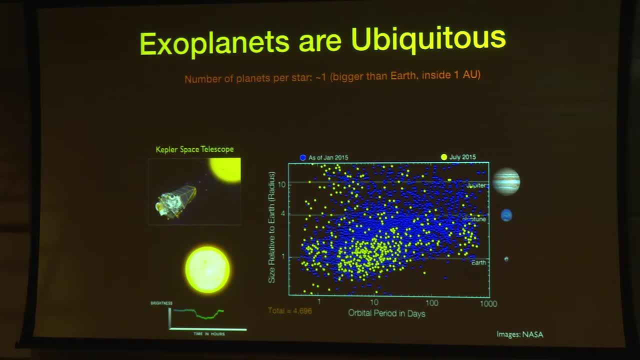 2 or 3.. So that means that somewhere between 30 and 50 percent of stars have planets and those that do commonly have more than one planet in this size range inside of 1 AU. We've done censuses outside of 1 AU, but they're less complete and they tend to be for bigger. 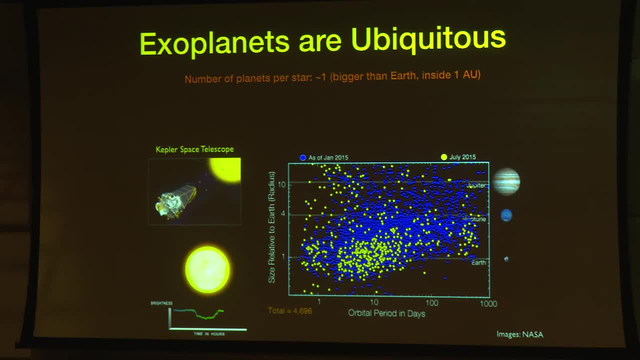 stars, so I'm not going to quote the numbers here. I think you get the general idea that planets are common. We've also done surveys for planets specifically Earth-like- and I say Earth-like with quotation marks, because what we're actually only able to measure to. 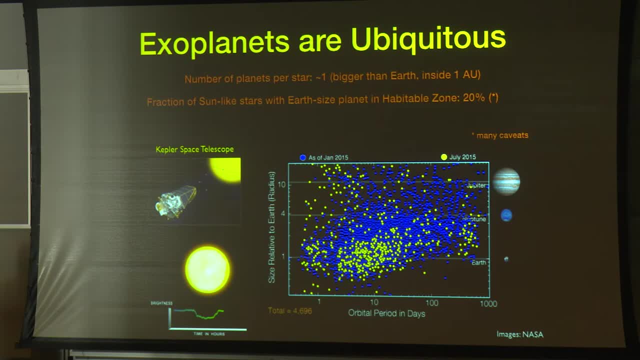 date is Earth size and the separation between the star and the planet, And we find that about 20 percent of planetary systems satisfy those two conditions: that you have the right size: approximately Earth size and approximately Earth distance in the so-called habitable. 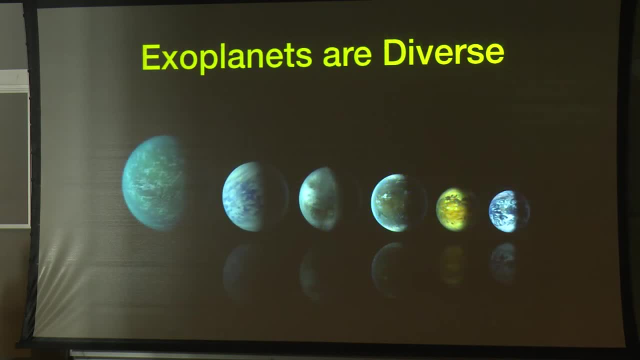 zone. We've also learned that planetary systems are diverse. We've discovered many new types of planetary systems, Perhaps most notably planets that are intermediate in size between the Earth and Neptune. We call these planets super Earths and sub Neptunes. These, in fact, represent the bulk of the planets. 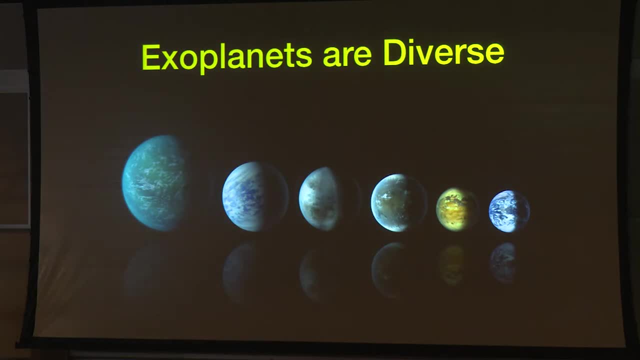 that have been discovered by the Kepler mission inside of 1 AU. We also see other types of planets not represented in the solar systems: highly eccentric planets, compact multi-planet systems with five or six planets all orbiting very close to one star. We see a lot of diversity. 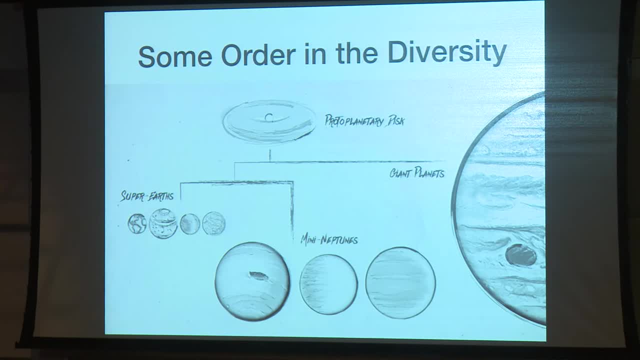 Thank you. Inside of that diversity we also see some order and we're starting to see that the broad set of planets inside of 1 AU can be grouped into types. So we see, for example, all planets we think descend from a protoplanetary disk, The first branch in this family tree of 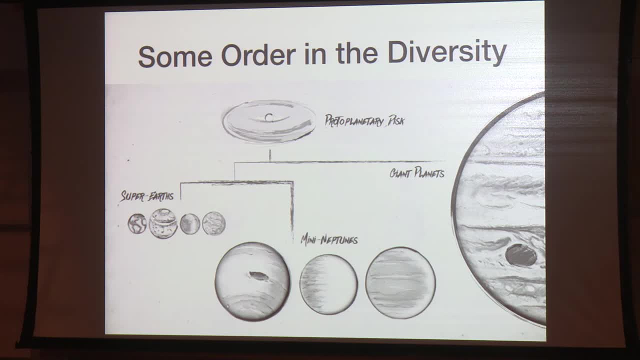 planets are the giant planets which are dominated by hydrogen and helium, likely with a rocky solid core of a few to 10 Earth masses. And then we see this other division of the mini-Neptunes which have of order 1% of their mass, hydrogen-helium, and the super Earths which are principally. 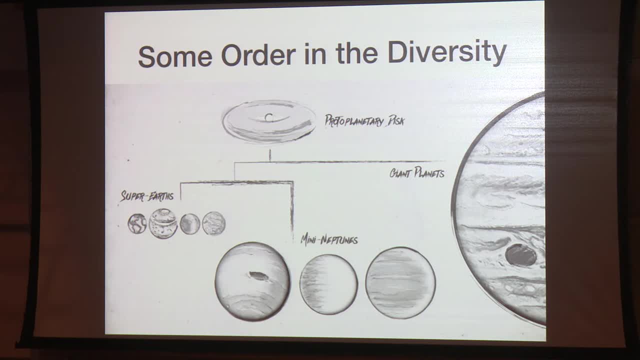 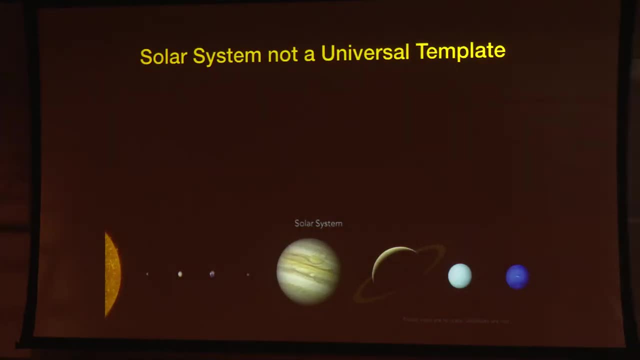 rocky. I think it's fair to say that the Earth is a small-size member of the super Earth family G quarters. What do I require? I'd also like to impress upon you the point that the solar system does not provide a universal template for planetary systems. 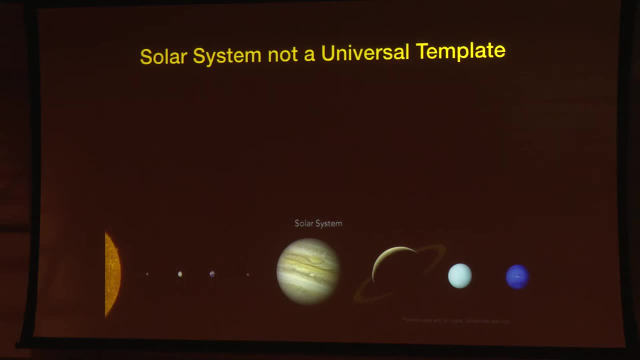 This is a mistake we kept making and interestingly, that's a mistake we kept making on this item. in the field of extrasolar planets. we kept looking for the solar system First. we were looking for Jupiter, because it's the easiest thing to find. 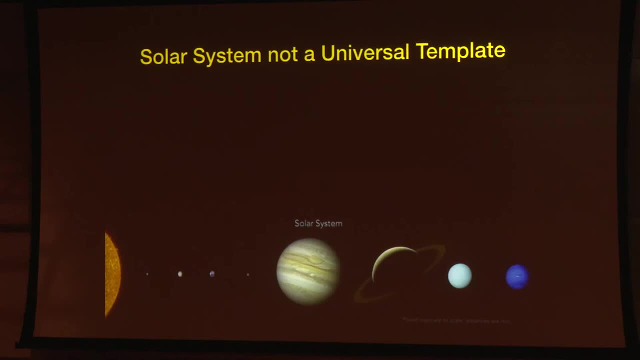 It's 5 AU, it's massive. We were surprised to find Jupiter and Saturn-sized planets orbiting very close to their host stars. We've been surprised over and over again by the architectures, the eccentricities and the mass distributions of planets. 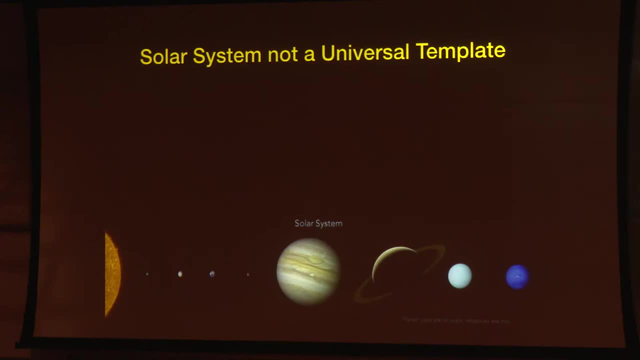 So we need to break out of our solar system-centric thinking. One example of a planetary system that does not obey the solar system architecture, which, by the way, is rocky planets, close in gas giants farther out and kind of fading away to the ice giants. 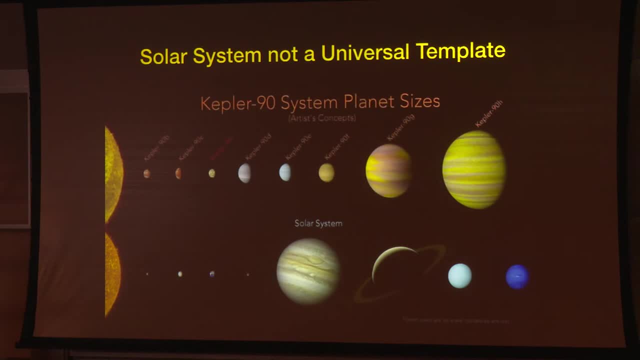 as you go to tens of AU. Here's a planetary system discovered by Kepler, much more compact than our solar system. It has six planets orbiting close in. These are all in the super-Earth and sub-Neptune regime and then two giant planets outside. 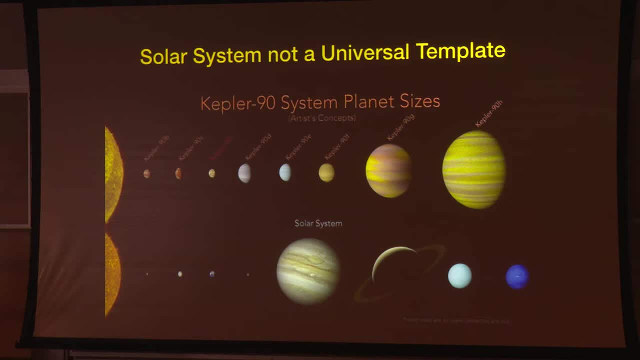 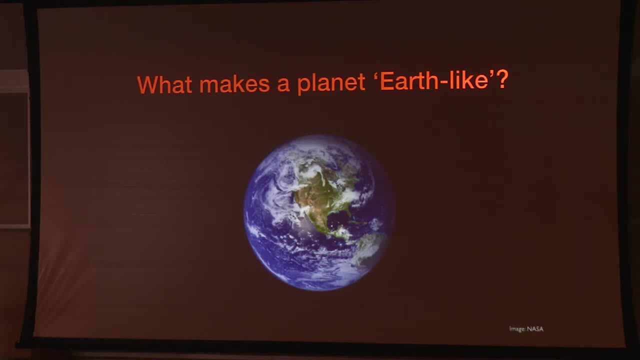 This is one of several non-super-Earth planets. This is one of several non-super-Earth planet solar system scenarios. So I'd like to close my portion of Jason's talk by describing a little bit about what I think makes a planet Earth-like. 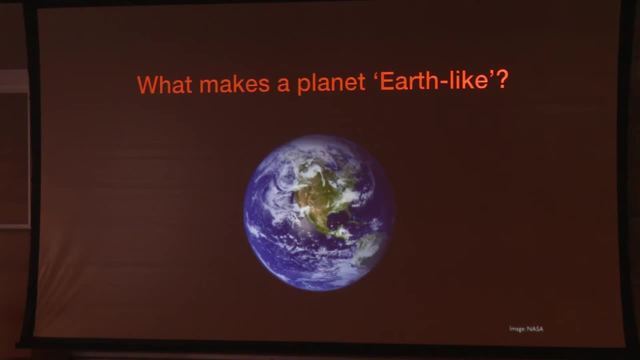 And in doing this I'm going to switch from, I'm going to not obey my own admonition to think outside the solar system. Let's think inside the solar system just for a moment, about what makes a planet Earth-like. Well, a planet, our Earth, certainly. 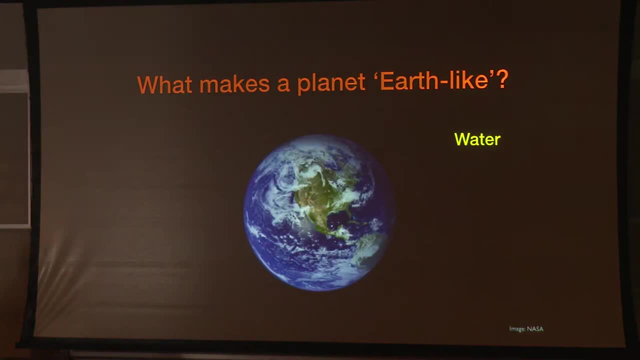 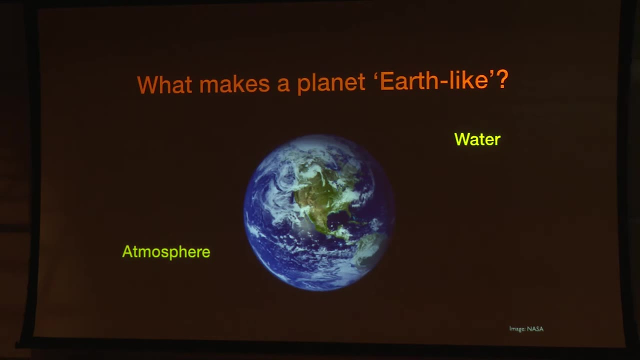 has water as one of its defining features. This water is in balance with an atmosphere that's also essential for life On the Earth. defining features are things like simple life, complex life, some of the finer things in life. Unfortunately, we're not able to actually measure. 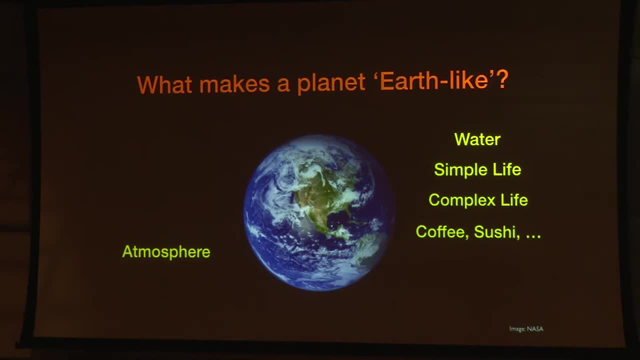 almost any of these. for extrasolar planets, The things that we can measure directly today are properties like the size, that is, the radius or the diameter, the mass, the bulk density. putting those together And the density gives us a clue to composition. 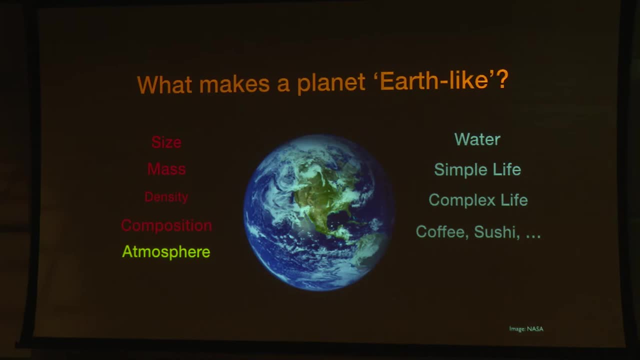 So I'm going to gray out the quantities on the right, at least for Earth-sized planets in the near term. We're not able to measure them. We have to make inferences based on the properties we can measure on the left. So that marks the end of what I wanted. 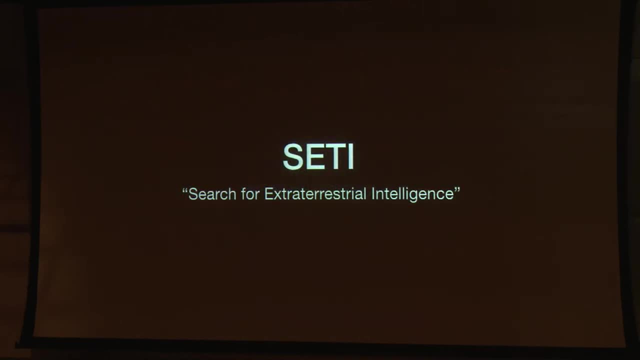 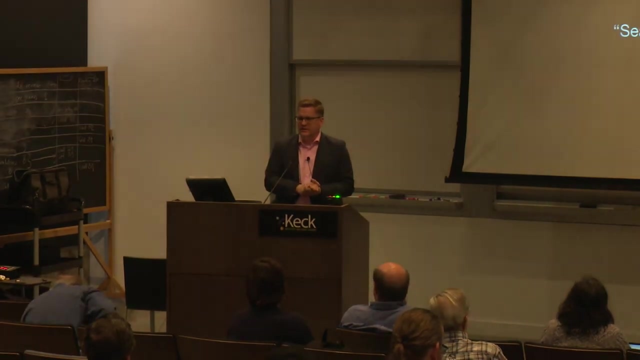 to say about extrasolar planets. I'd like to now introduce Sophia Shaikh. Sophia is a PhD candidate at Penn State, Penn State University. She works with Jason Wright. Sophia is a graduate of the University of California, Berkeley, where she received degrees. 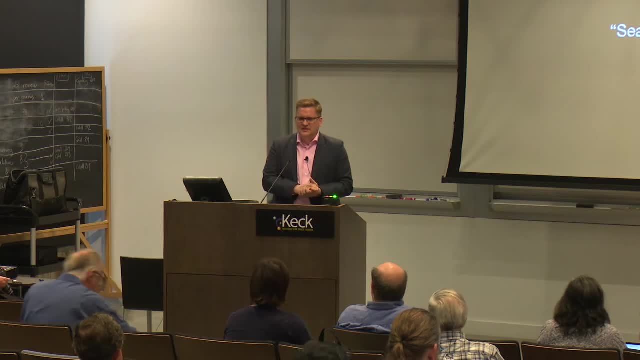 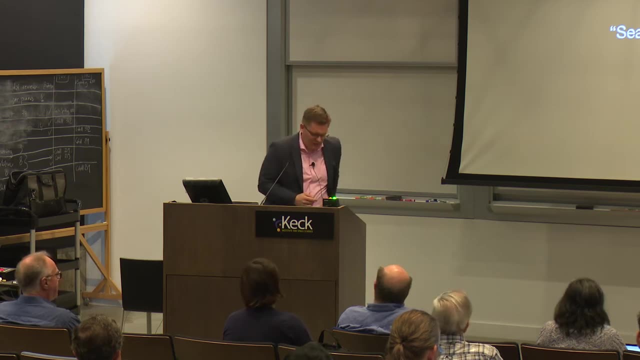 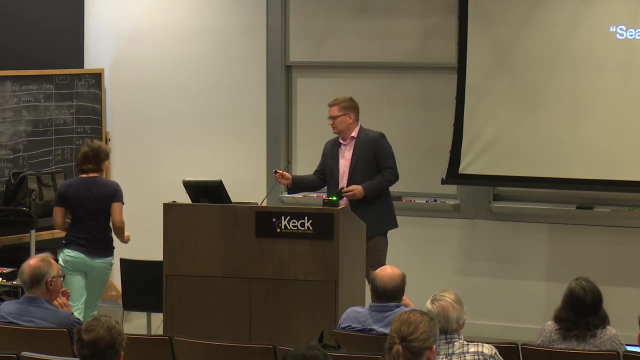 in physics and astrophysics. Sophia is, I think, part of the great resurgence in the last few years of SETI and the search for technosignatures. So, without any more, let me hand it over to Sophia. All right, thank you, Andrew. 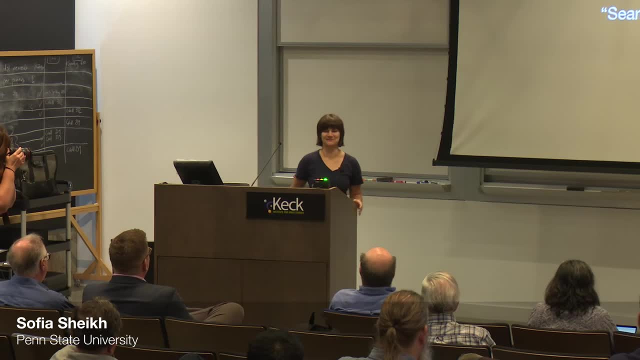 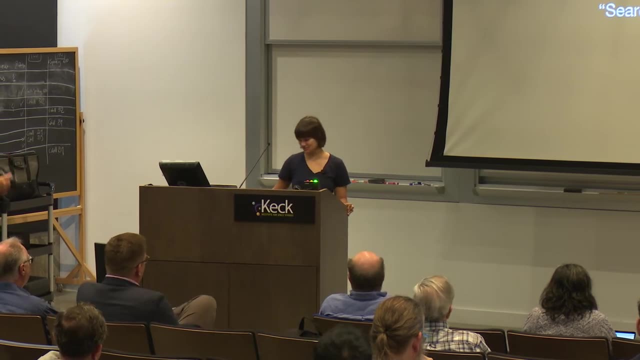 And I'm really glad to be here. A little surprised to be up at the front of the room today, but there you are And I'm going to be talking about SETI and the search for technosignatures. And to kick that off, when we're discussing these topics, 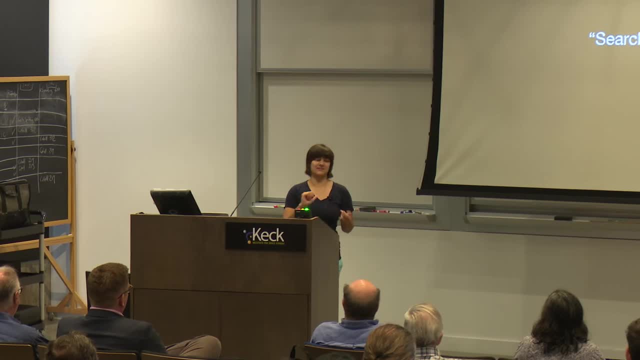 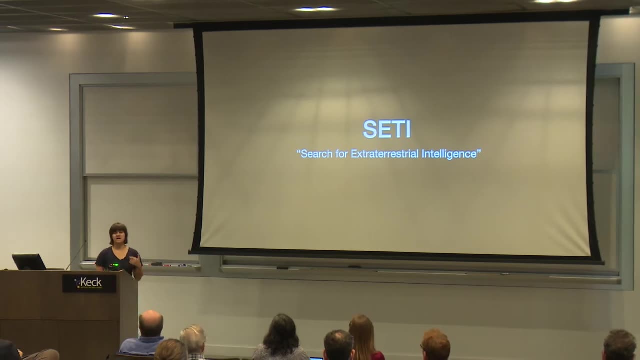 because the field of SETI has been small, it's very interdisciplinary and it's kind of had a spotty history of funding and politics that are kind of tied up with it. the language that we use to talk about the field is similarly kind of fragmented. 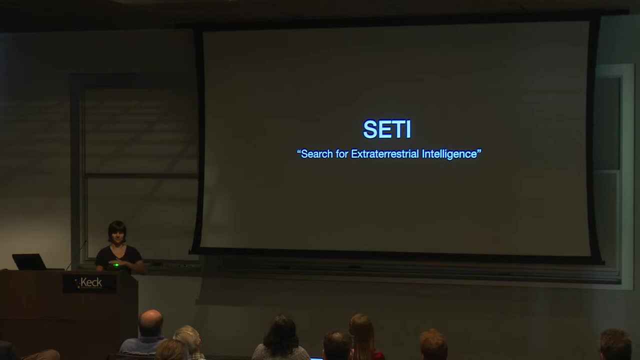 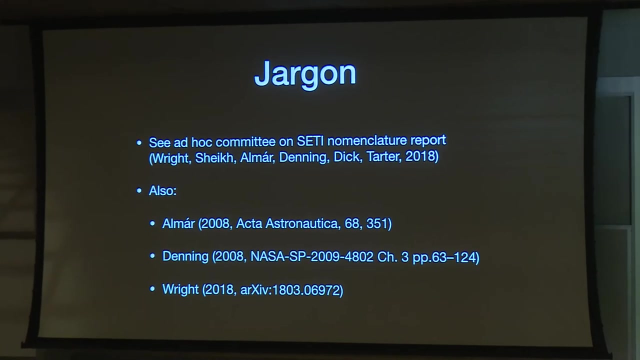 And so the first thing I want to do is define sort of a universal jargon that we can use and talk about, so we're all on the same page, And the definitions and fundamentals that I'm going to talk about are described in the ad hoc committee on SETI nomenclature report that 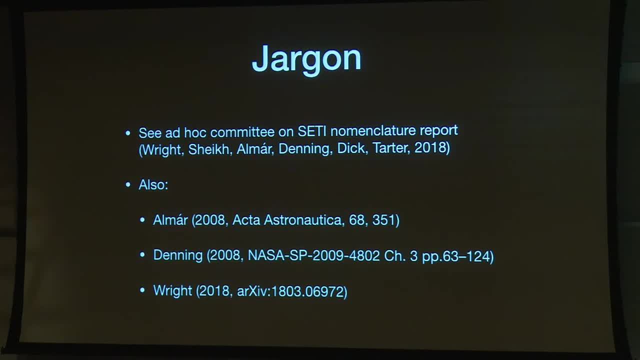 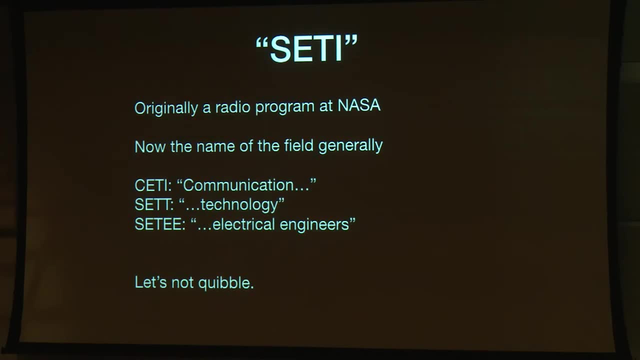 was put together last year. So if you're curious about this, here are some references and you'll be able to access them And you'll be able to access the slides later. So first of all, starting with SETI itself originally, 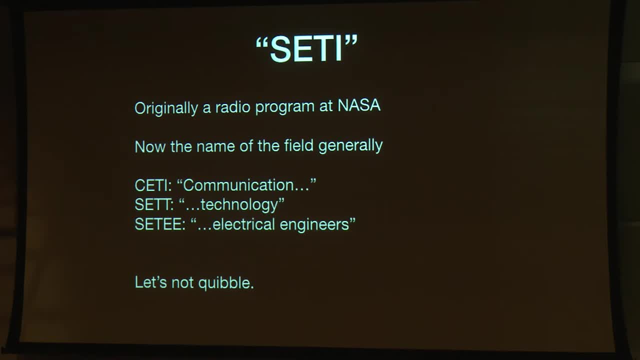 the name, which is an acronym for Search for Extraterrestrial Intelligence, referred to a radio observing program at NASA. So it was specifically for one scientific program And since then it has broadened to be the entire subfield of looking for extraterrestrial. 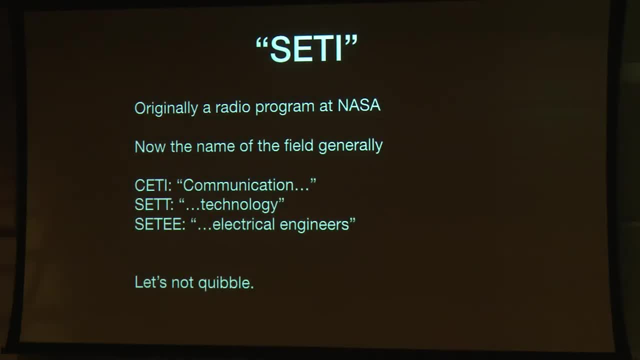 intelligence, intelligence beyond our solar system. So in addition to the standard SETI, there are other variants that show up in the literature, including SETI with a C standing for Communication with Extraterrestrial Intelligence, SETT- Search for Extraterrestrial Technology. 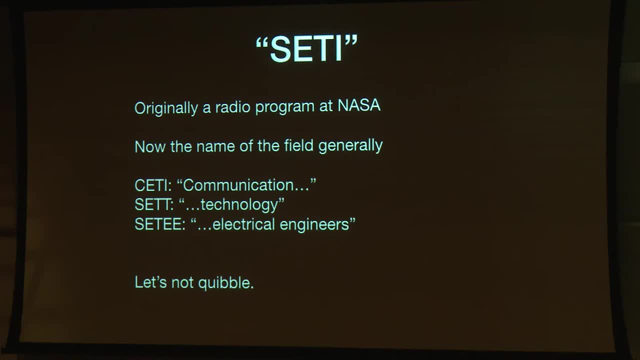 because, in essence, we're not searching for the intelligence, We're searching for products of that intelligence. And SETI with two Es, Search for Extraterrestrial Electrical Engineers- because, again, we're not really searching for the intelligence itself, but what that intelligence produces. 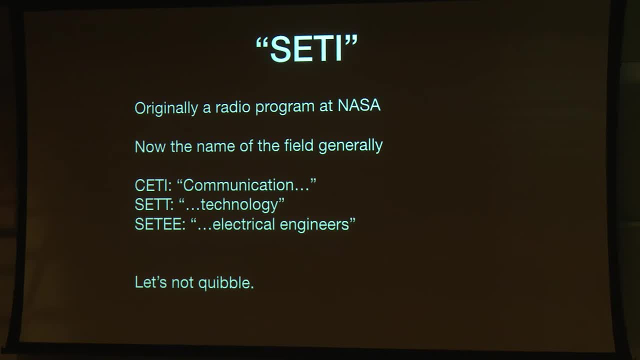 And most of that so far has been searched for electromagnetic signals. So all of these exist, You will see them, But for the purposes of this talk and conference, we'll be using SETI primarily, And not only will we be using SETI. 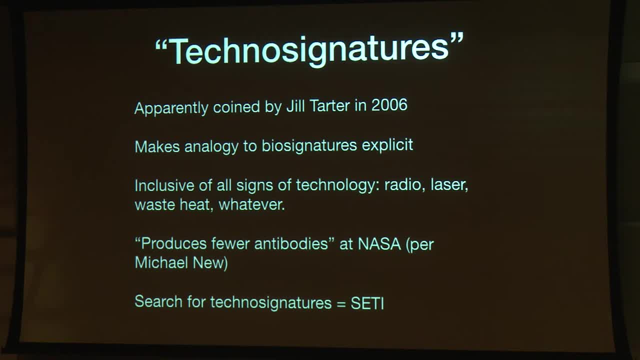 we'll also be using technosignatures, which is a more recent term As far as we can tell. tracing the term back, it was coined by Jill Tarter in 2006.. And it's nice because it makes the analogy to biosignatures explicit. 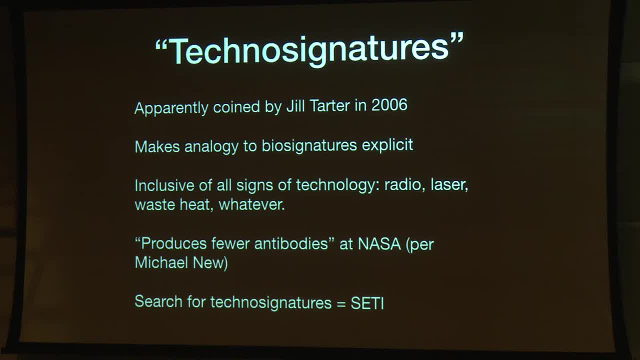 The search for biosignatures is a very big thrust in astrobiology right now, especially at NASA, And so kind of making that analogy and comparison to really show how the two fields can work together is important. Technosignatures is a nice term because it's 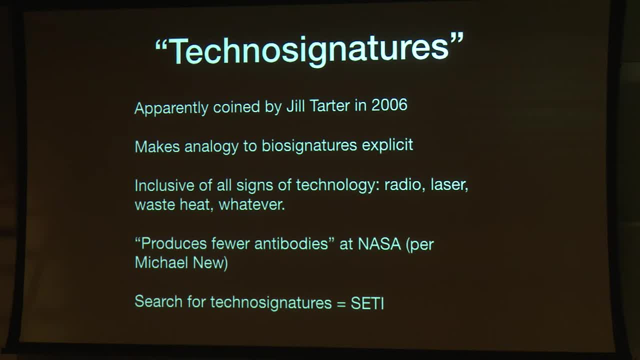 inclusive of all signs of technology. So this includes kind of the traditional SETI radio searches but also optical and infrared search, searches for lasers, searches for waste heat and other artifacts. All of them are included under this umbrella of technosignatures. 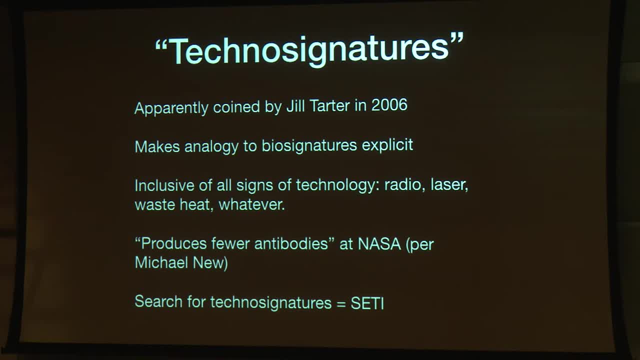 As per Michael New at NASA, the term technosignature or saying search for technosignatures produces fewer antibodies at NASA. As I sort of alluded to on the first slide, the term SETI and the idea of SETI. 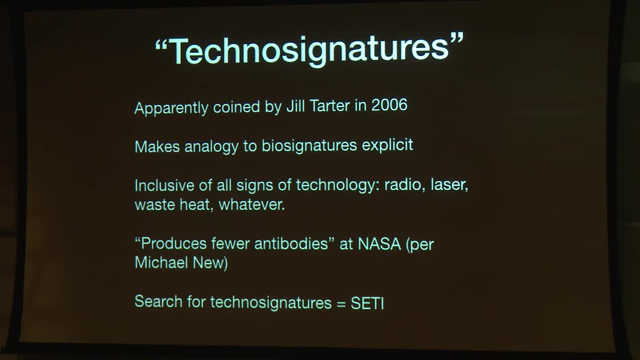 has kind of gone through a rocky history of what people think it is, What it actually is and how funding and political landscapes have worked over the years. And so, even though SETI is the search for technosignatures- and when we say search for technosignatures we mean SETI- 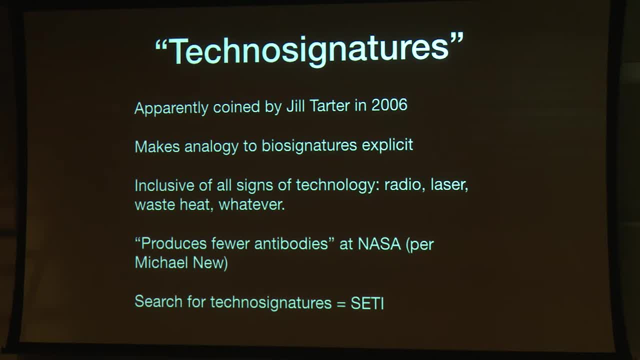 in general, technosignatures is more of a term that's coming in vogue now because all of these reasons, but also to kind of distance itself from that rocky history of the term SETI. So these are terms you should be using and should know. 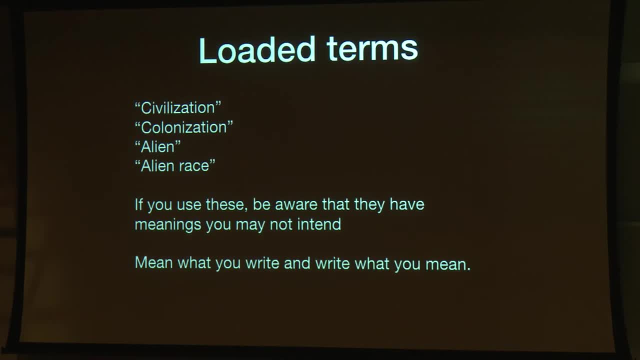 how to use Terms to kind of avoid- although sometimes they sort of slip into your speech- are things like civilization, colonization, alien or alien race. If you use these terms, just be aware that they have connotations and meanings you might not intend. 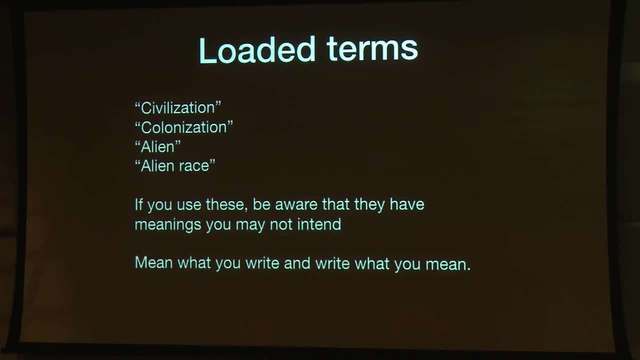 And also be aware that a lot of these terms have specific meanings in other fields. So if you're talking to anthropologists, you can't just throw around the word civilization without realizing that they're going to I think think you're talking about something very specific. 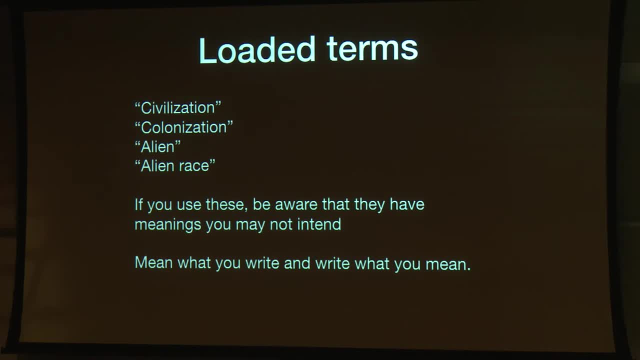 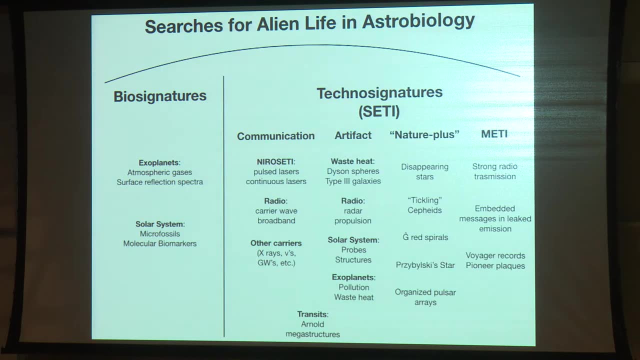 that you might not be intending. So mean what you write. write what you mean To kind of give you an idea of how this fits into astrobiology as a whole. we have this diagram we've put together and I'm not going to go through. 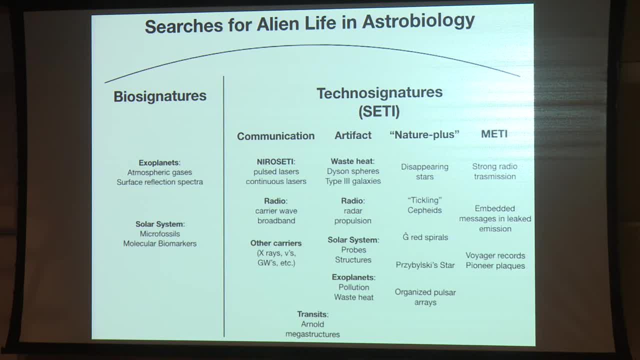 every category on here, but the important thing is that searches for life in astrobiology are kind of an umbrella blanket, and then under that you have searches for biosignatures, and that includes things like look for a, looking for gases in exoplanet atmospheres. 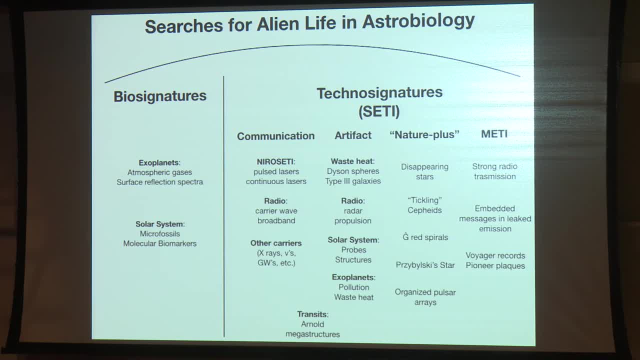 looking at their reflection spectra and in the solar system looking for microfossils, biomarkers, isotopic signatures, things like that. So that's kind of traditional biosignature research. And then, just as another side of the coin, analogously, 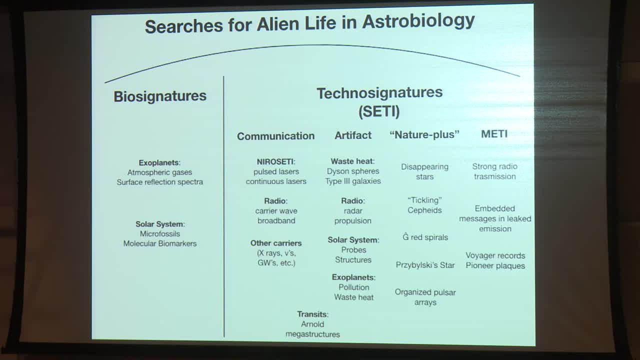 you have technosignatures or SETI, And underneath that umbrella you have even more subcategories. So things like communication SETI, looking for intentional communications in the radio, in the infrared, in the optical and maybe in other carriers. 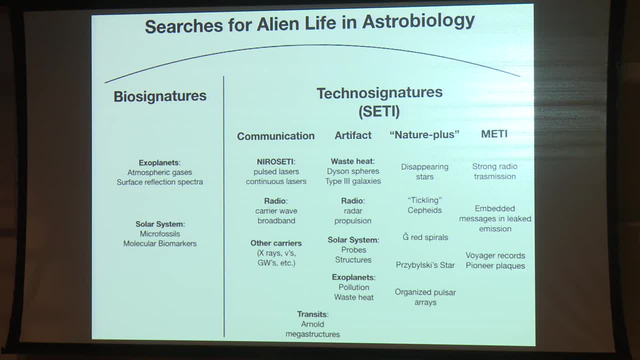 Artifact, SETI, which has to do with looking for products of technology that are not meant for communication. So this can be things like looking for waste heat, looking for radio leakage or unintentional radio signals, looking for artifacts within the solar system or looking at exoplanets for changes that technology can produce. 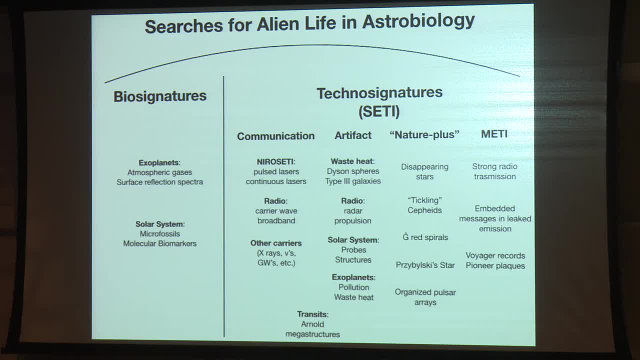 in their atmospheres, for example. So the third category. there is a little bit more out there. We call it Nature Plus, And that's something that includes anything that is astrophysically an anomaly or interesting that we wouldn't be able to explain without invoking technology. 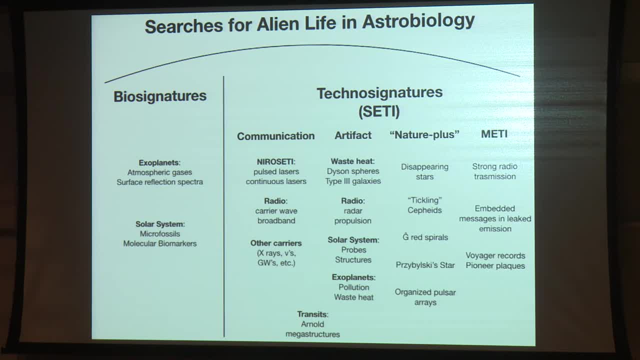 So stars that disappear, stars with very strange spectra pulsars that are somehow organized in arrays, things like that. And finally, for completeness, we include METI as a final branch. So that's the first category, So the third category. there is a little bit more out there. 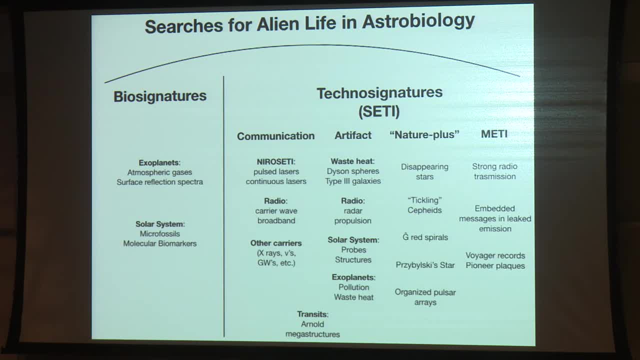 We call it Nature Plus, And this is short for Messaging Extraterrestrial Intelligence. It is controversial, And the idea behind METI is that, in order to discover if anything's out there, we have to elicit a signal, And so this could be via strong radio transmissions. 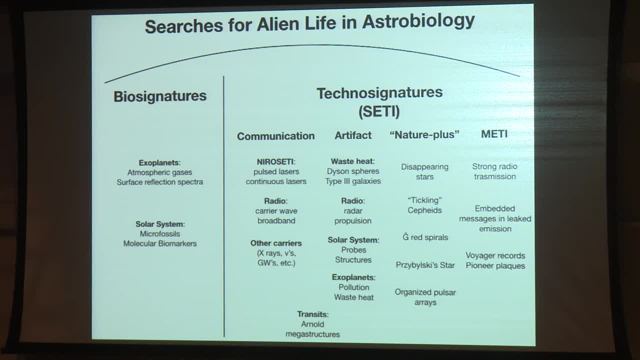 and it could be via things that are actual physical artifacts that we send out, such as the Voyager records or the Pioneer plaques. So there are a lot of different ways to come up with these things, So we're going to talk a little bit more about how we come at this problem. 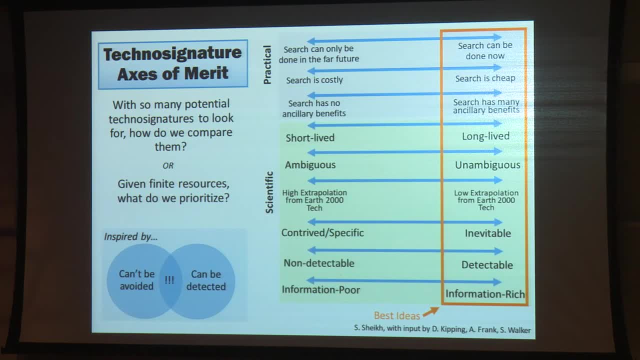 And one of the things that you have to think about is how to compare these projects that have entirely different methods, entirely different goals. What you're searching for is different, How you're searching for it's different. So how do you compare two searches on a level playing field? 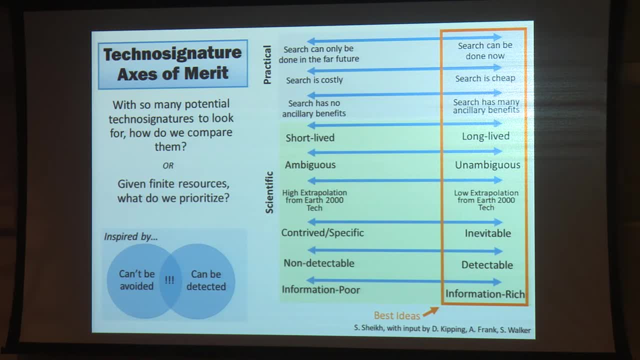 And to that end we have put together these axes of merit. So there are nine different axes on which you can place any technosignature search. So the first first axis is merit. The first few axes are things that come up in almost any astronomical campaign. 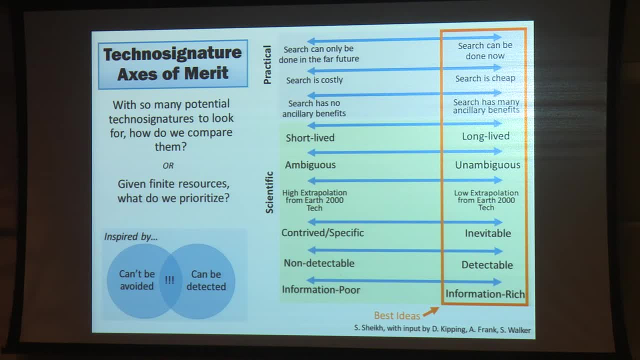 You would prefer searches that you can do right now. with technology, we have to searches that would require instruments that we haven't built yet. We prefer cheap searches to expensive ones. of course, We prefer searches that have ancillary science benefits to ones that don't. 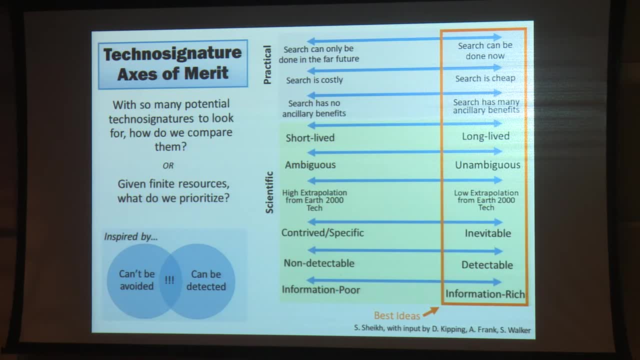 So when you're designing a SETI search, even if you don't find any signs of extraterrestrial nature, you're not going to be able to find any signs of any sort of scientific validity. Or, for example, if you're trying to use scientific 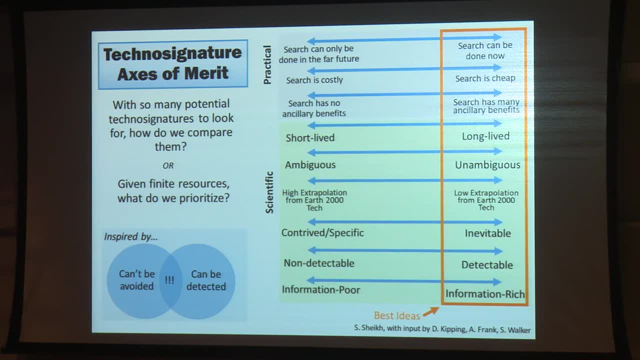 or scientific intelligence. your search should provide something that is of value to the scientific community, ideally other than just an upper limit, And so you prioritize searches that have other benefits, And that could be things that you find astrophysically, And it could be methods that you develop or different software that you can use in other places. 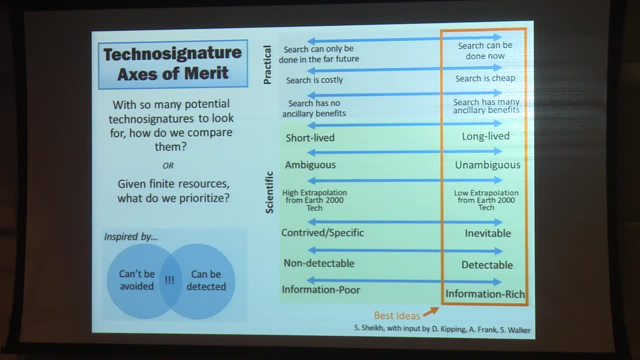 Then, kind of moving on to scientific axes, You would prefer a signal that is long lived to one that is short lived, to give you a better chance of being present than a more long-lived one. So that's that being able to detect it even at low frequency in the universe. 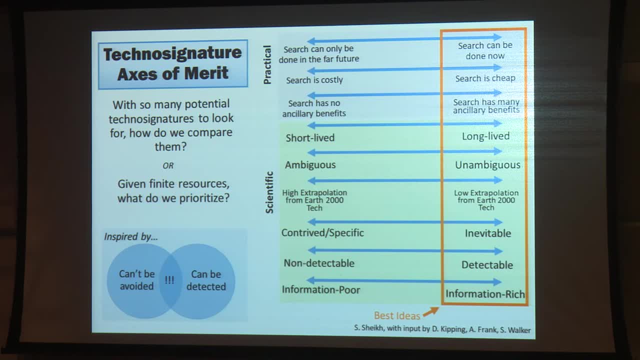 You prefer a signal that is unambiguously a sign of technology to something that has natural confounders, And this is why one of the main reasons why radio SETI has been so popular for so long is the things that radio SETI is searching for don't have any astrophysical sources, as 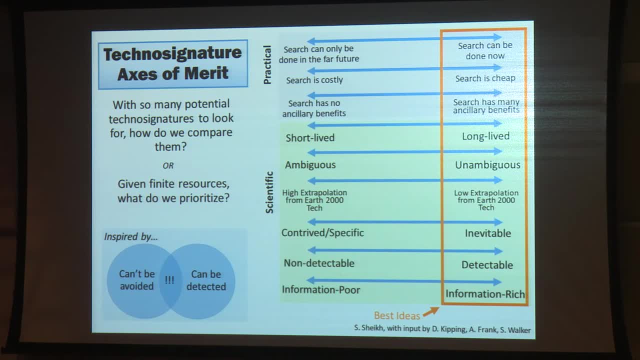 far as we know. So if we were to find it, it would be an unambiguous sign of technology. The next axis there is how much extrapolation we would need from our technology to be able to produce the signature we are looking for. So you prefer something that we know is possible with technology to something that we theorize. 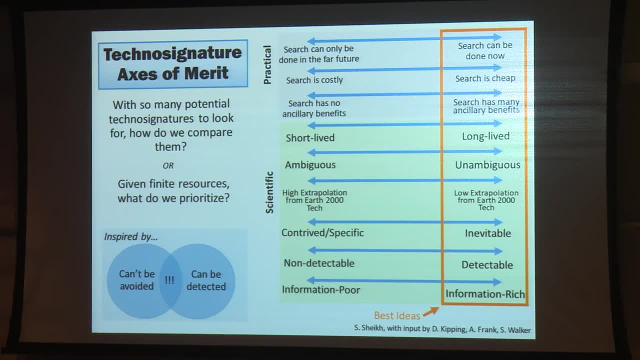 could be possible. For example, we know we can send narrow band radio signals. We don't know if it's possible to build a Dyson sphere. We prefer inevitable signatures to those that are very specific. So if you have signals, some signature. that seems to be an inevitable product of a civilization's development. 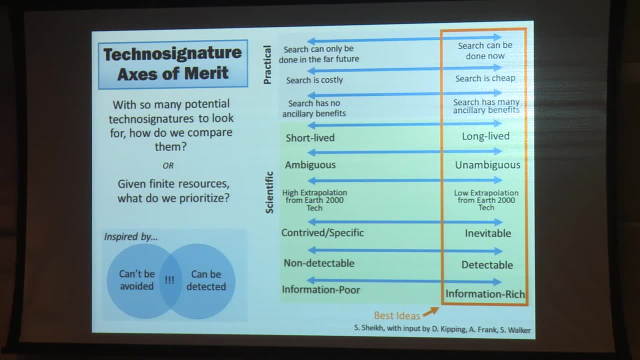 So no matter where in the universe it happens, you'll always get the signature. You would prefer that to a signature, such as looking for a very specific chemical from plastics in an atmosphere or something like that. Then, kind of the obvious one, you prefer a signature. 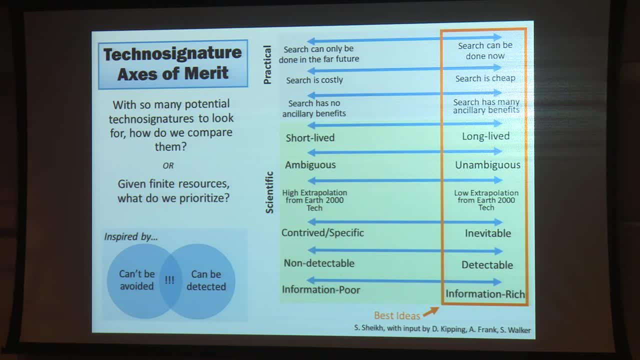 that is easily detectable at high signal-to-noise to something that would be borderline detectable or very difficult to detect. And the last one: there is information rich versus information poor, So it would be nice that if we did make a detection we could tell something about. 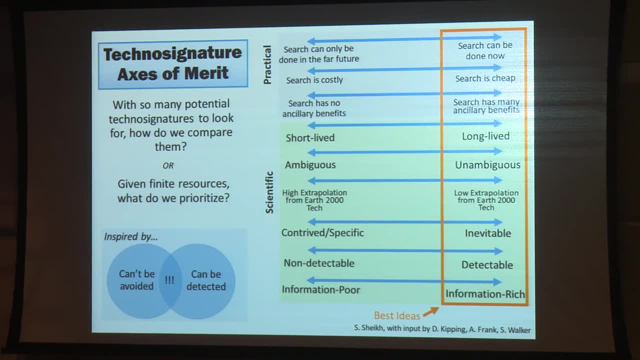 the technology or the species that created it, versus only being able to know: yes or no, is there another intelligence in the galaxy or in the universe? So these are things to keep in mind that you can apply to almost any technosignature search, And I'll admit. 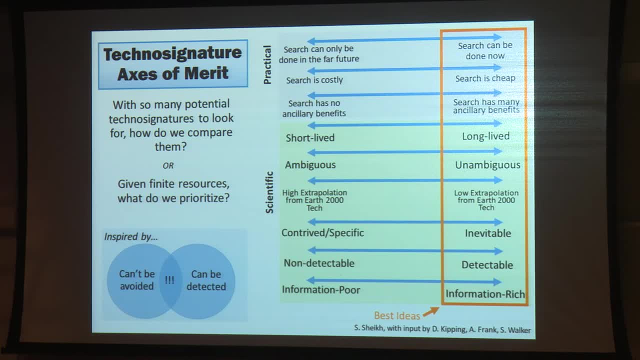 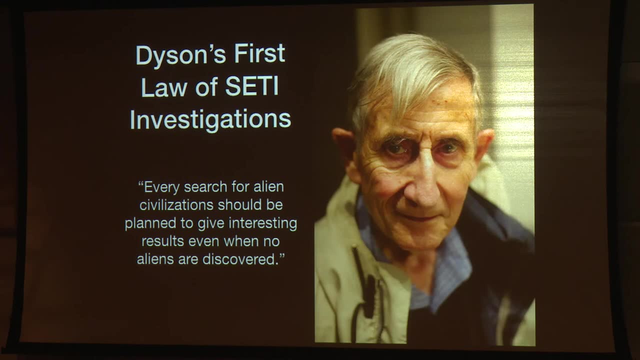 these are not Kind of novel thoughts. These have been discussed before in many different contexts And in fact one of those axes lines up with Freeman Dyson's first law of steady investigations, which is that every search for alien civilizations should be planned to give interesting results. 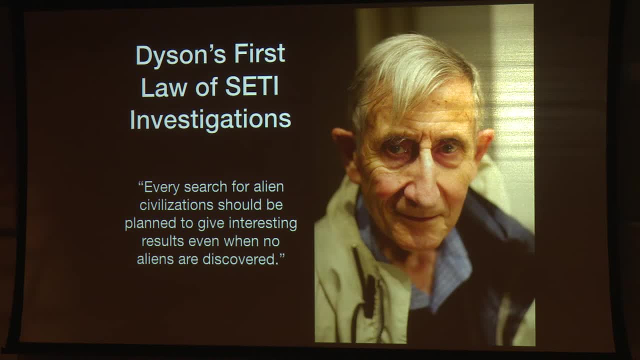 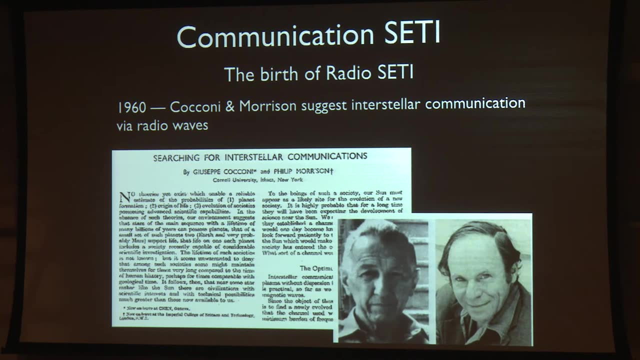 even when no aliens are discovered. So now what I'm going to do is jump into some of those branches I talked about before and just give you a little bit of a history of what's been done in each of these. So first of all, communication, SETI and the birth of radio SETI, And this occurred in 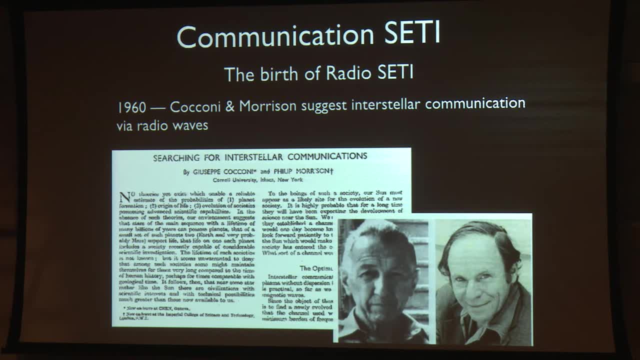 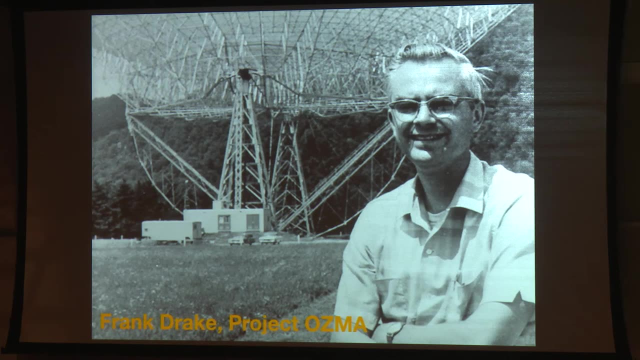 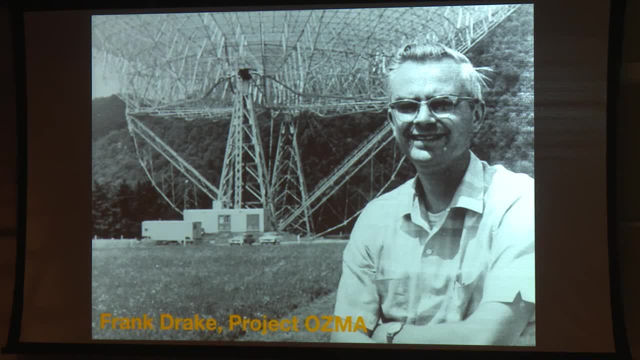 And it was a research that was done in the first place. And it was a research that was done in the first place And even though that project targeted only a couple of stars nearby the Earth, a few decades later we've expanded upon that idea and we have projects like Breakthrough. 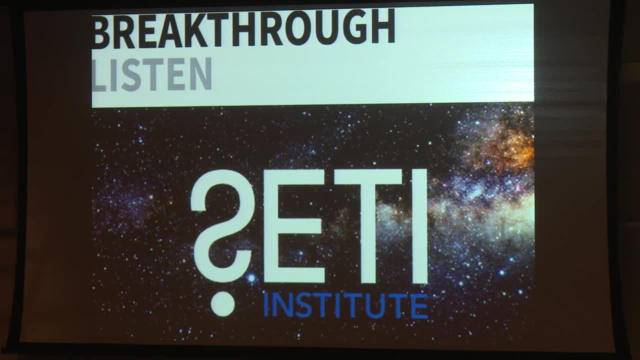 Listen and instruments like the Allen Telescope Array at the SETI Institute that are dedicated instruments and dedicated projects searching thousands and eventually millions of targets. So radio SETI has kind of experienced this exponential growth orders of magnitude. more parameter space is being searched now than was able to do in the first place, And it's 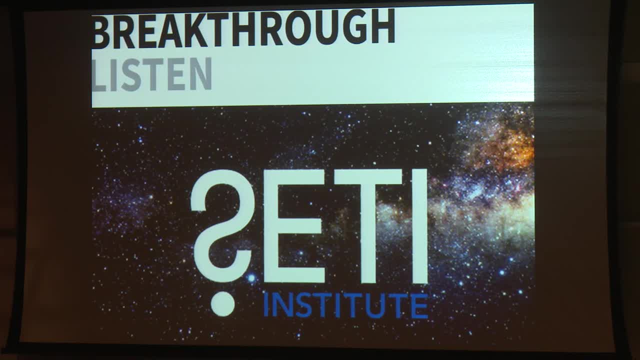 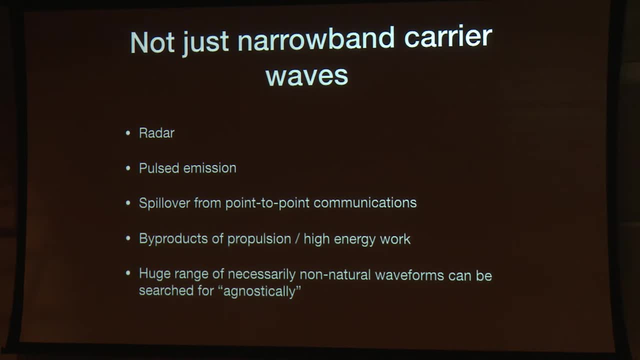 also expanding out in the types of signals that we're looking for. So you'll hear a lot about narrowband carrier waves, And that's the idea that if you send a signal that's very, very narrow in frequency range, then there's no astrophysical source. we know that. 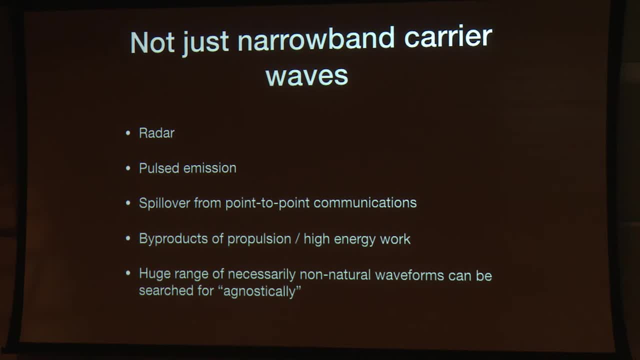 can do that And you have to be looking at something artificial. So that logic has been used for a long time. But you can also, instead of looking for an intentional narrowband signal, Look for maybe unintentional leakage from radar, or, instead of looking for a signal, that's constant in time. look for something that's pulsed. Look for spillover from point to point communications that aren't supposed to include us, Looking for radio emission that's just a byproduct of some propulsion or high energy work, Or maybe not even thinking about these really narrow signals, but any signal type that you. 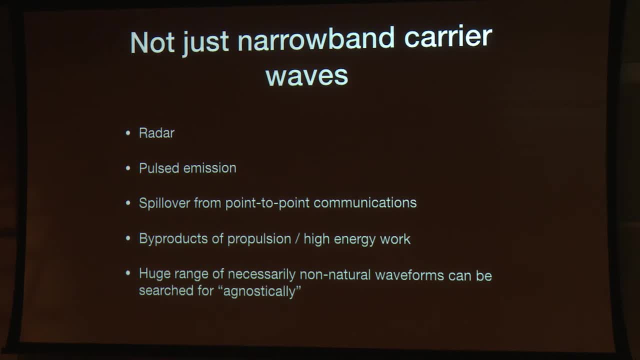 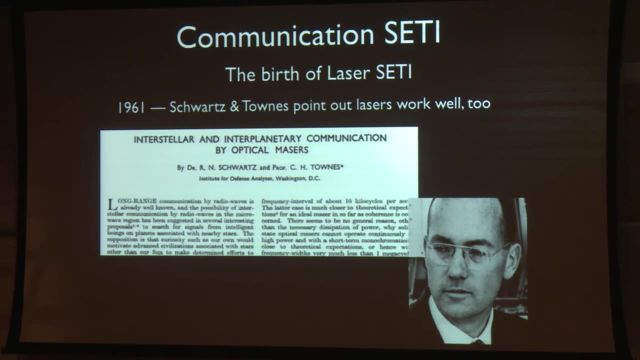 wouldn't expect astrophysically. So we need a way to look for waveforms agnostically, without assuming their shape or modulation. So the flip side: you have radio searches and you also have optical searches for lasers, And so this was proposed. you'll notice around the same time, within a year of the first. 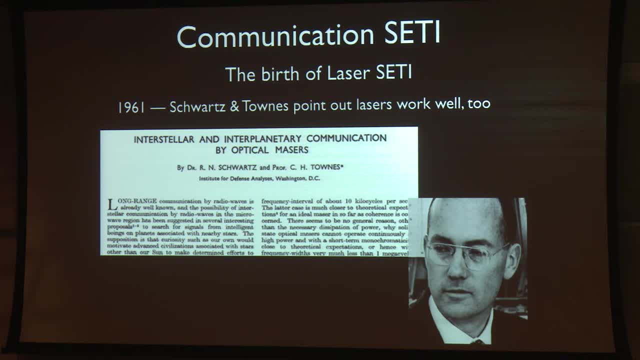 search by Frank Drake, And it was proposed by Schwartz and Townes, And Townes you'll recognize as the inventor of the laser. So he realized the consequences of his discovery very soon after making it, which is that lasers could be used for interplanetary and even interstellar communication. 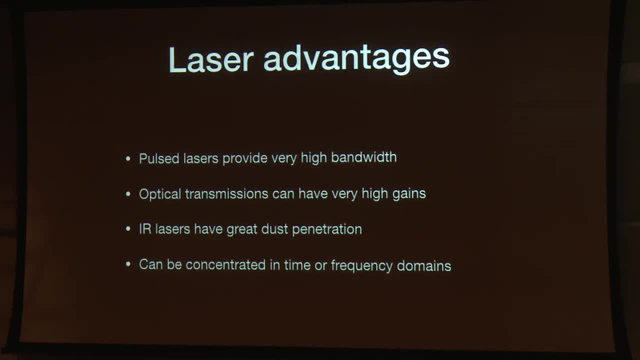 And there are a lot of advantages to lasers that you don't get with normal broadband optical signals. So pulsed lasers give you a very high bandwidth, Your optical transmissions can have very high gains And infrared lasers have great dust patterns. And infrared lasers have great dust patterns. 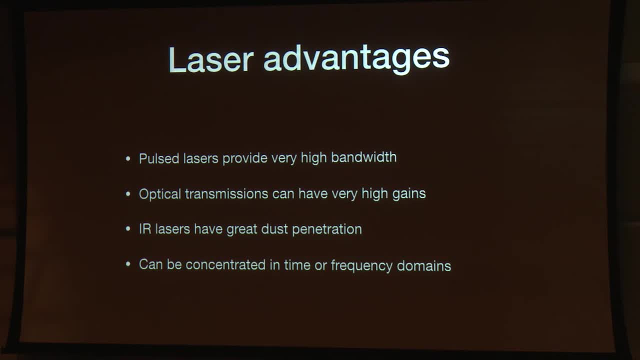 And infrared lasers have great dust penetration, which is very nice, because usually if you're trying to send optical signals you have to deal with dust extinction, And lasers can be concentrated in either time or frequency domains. So really narrow in time signals that last maybe nanoseconds, or really narrow in frequency. 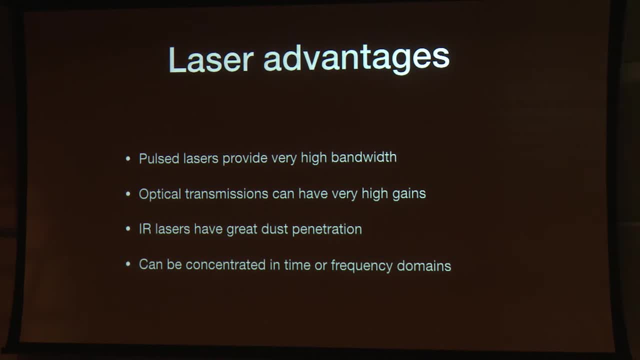 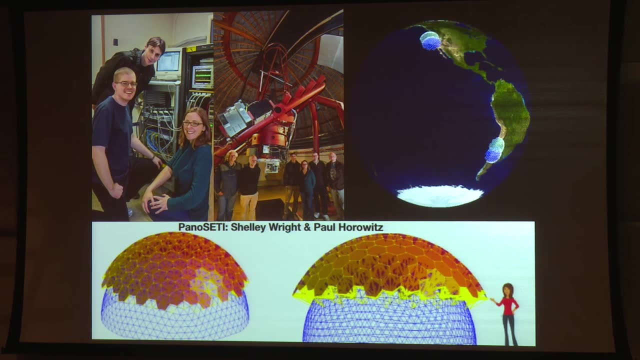 signals are both good ways to transmit information and signals via lasers. So I'm just going to highlight one project that is a current laser SETI project, which is PanoSETI- PanoSETI, And that's the brainchild of Shelley Wright and Paul Horowitz. 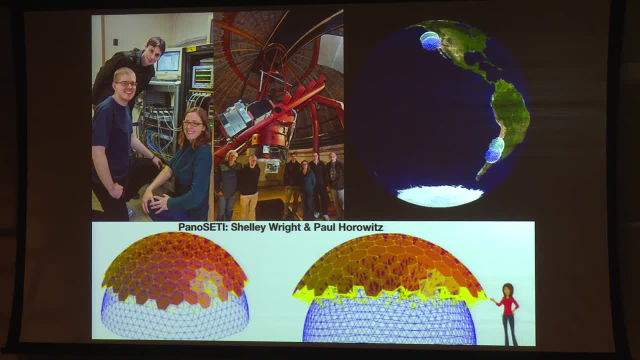 And PanoSETI is interesting for many reasons, but one of the ones I want to highlight is that it's leading towards all-sky, all-the-time SETI, So being able to look in all directions simultaneously and be able to have that observation going. 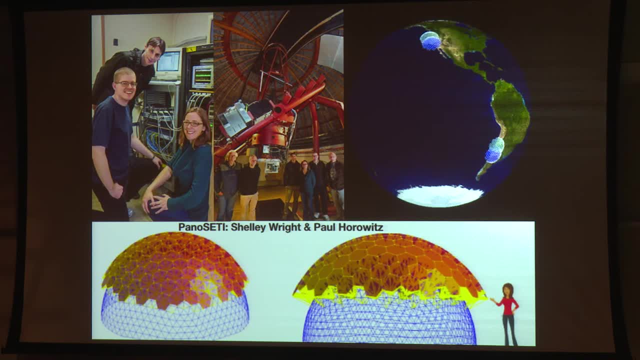 for a long consecutive time. So we can have this baseline of observations that we've never had in the past, And the way that they're going to accomplish this is with this really neat fliesight, And that's something that's kind of in the development stages right now. 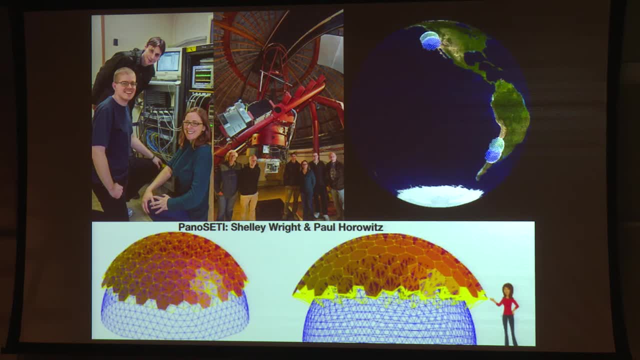 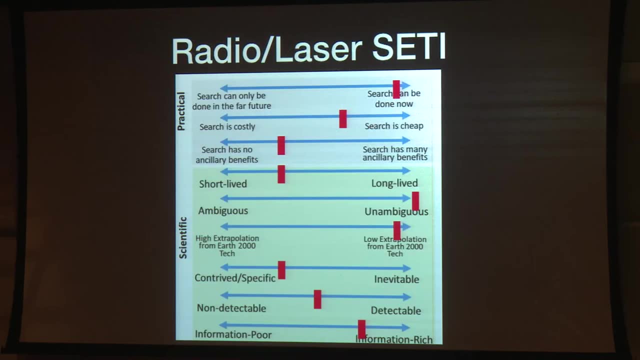 But if you're looking for more information on optical and infrared laser searches, I would highly recommend to look at their instrumental papers. So I'm not going to go through all of this, but this is kind of a qualitative idea of where radio and laser SETI fall on these nine axes. 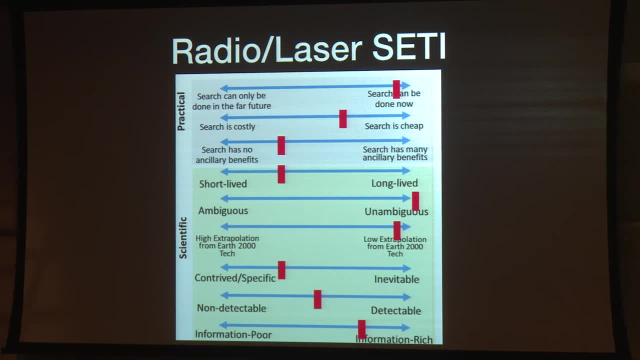 One of the great benefits to these searches is that we can do them now. We have the technology. We've been doing it for decades. If we find something from a laser search or from a radio search, it should be unambiguous: which is nice. There aren't any natural confounders for these really narrow wavelength signals. We don't require any extrapolation from what we can do right now. We have the technological capability to send these signals, so we don't have to assume any technology we haven't yet invented on Earth. 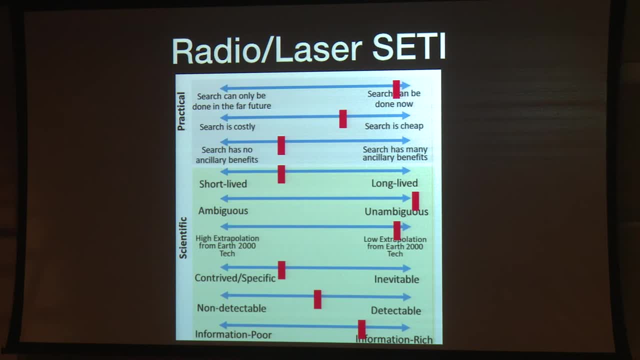 So that's that, And they could be pretty information-rich Kind of. the downsides of searches like this are that you often don't have that many ancillary benefits because you're looking for signals that are purposefully not astrophysical, so you're not going to find astrophysical things when you perform them. 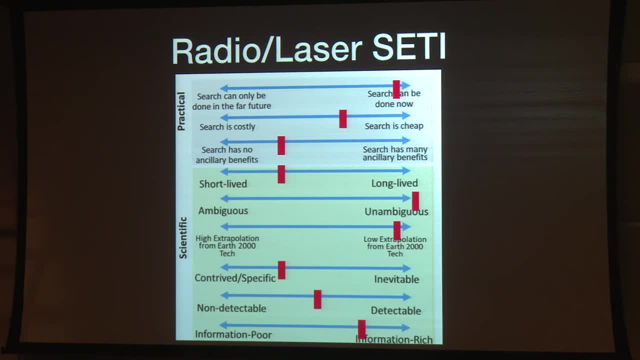 The signals we're looking for could be pretty short-lived, depending on what you assume about the transmitter, And it is kind of a contrived situation, Especially, Especially in communication, SETI, where a signal is being sent to us, You have to make the assumption that someone is sending a signal to us, which is a pretty 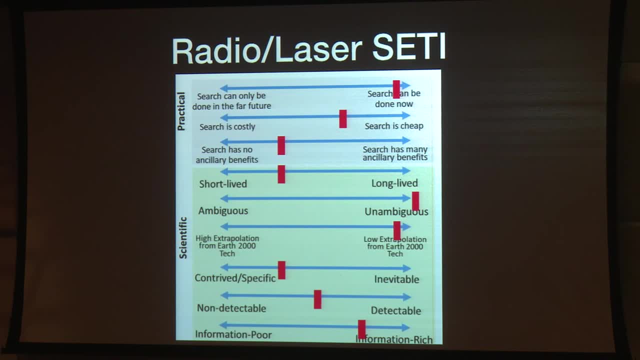 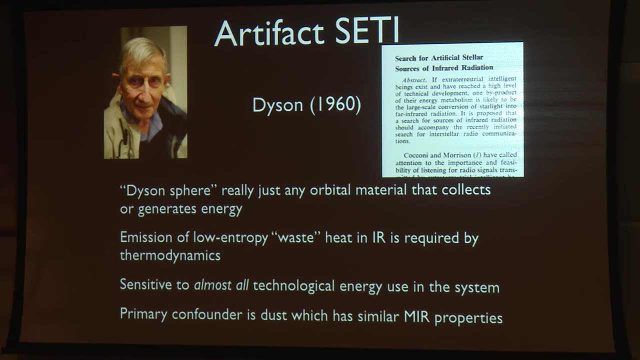 big initial bar. So now we're going to move from communication SETI to artifact SETI And that's kind of the polar opposite in many ways. So artifact SETI- you'll notice the year 1960, again started around the same time. 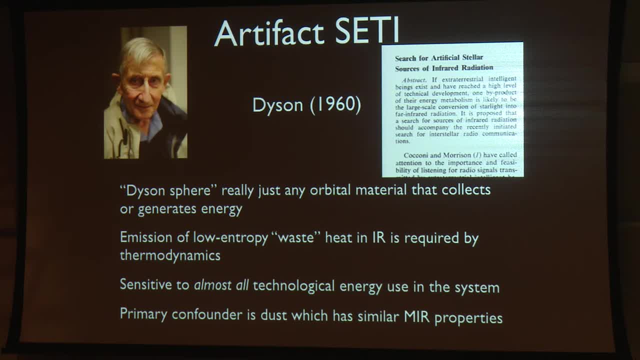 And Freeman Dyson came up with this idea That You have orbital material that collects or generates energy. You're going to have some sort of entropic waste heat signature from it, And that has become known in popular culture as a Dyson sphere, although picturing it as 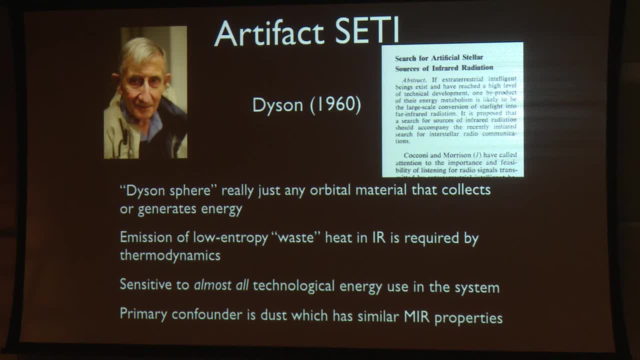 a solid sphere is sort of a misnomer, And the more generalized form basically just says: whenever you're generating or collecting large amounts of energy, you're going to be producing this infrared waste heat, And that means you don't care about exact amounts of energy. 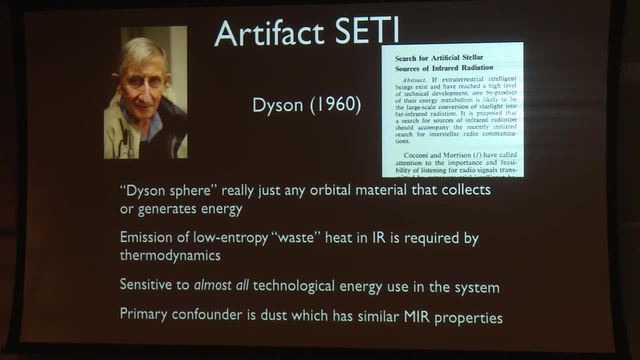 You're going to be producing this infrared waste heat, And that means you don't care about exact amounts of energy. If you don't know exactly what the structure is, or what it's made of or what it was built for, you're still going to get the waste heat. 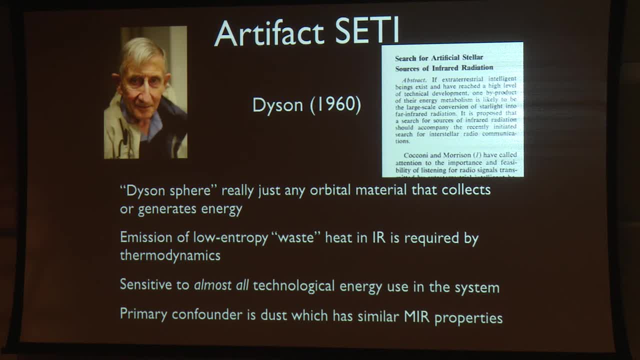 So it would be sensitive to almost all technological energy use in the solar system. The problem with this is, if you're looking for excesses in the infrared coming from Dyson spheres, you're going to find excesses in the infrared coming from dust. 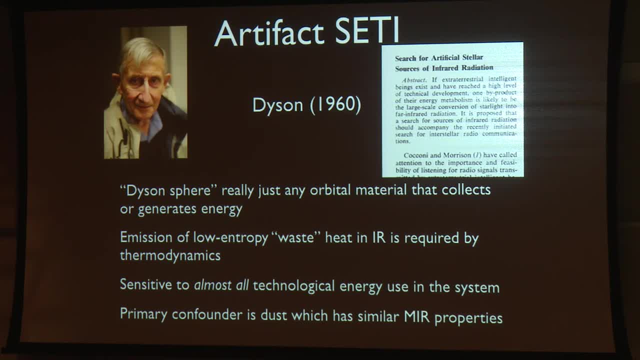 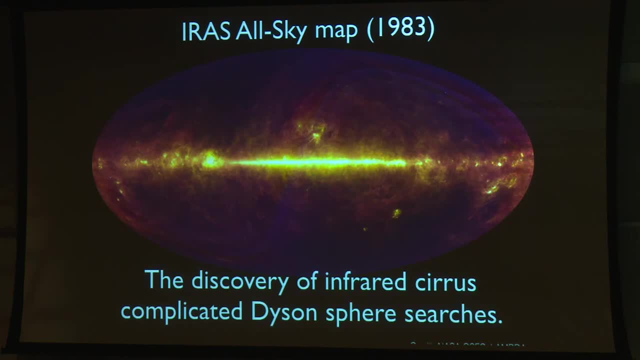 So you have to deal with that natural confounder. And complicating this even more, 20 years later we had IRAS, creating an all-terrain, all-sky map in the infrared. And not only do you have to deal with dust in protoplanetary disks and dust that is circumstellar. 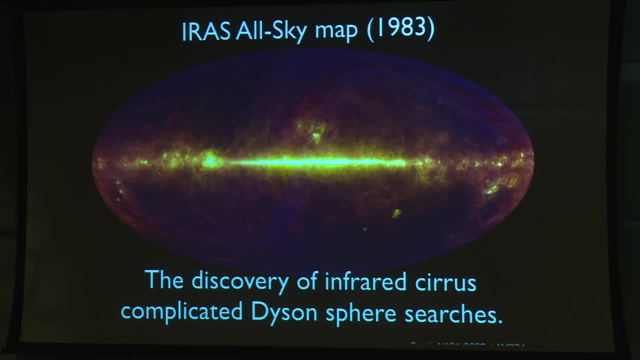 you also have to deal with just the infrared cirrus, And so you can see the galaxy in the midplane here, which is glowing very brightly in infrared, But there's dust that goes pretty far off that midplane too in these kind of wispy. 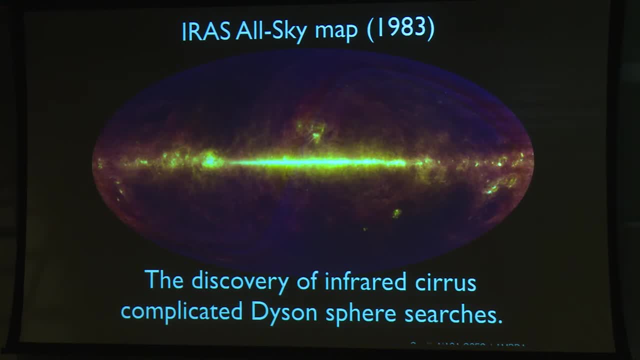 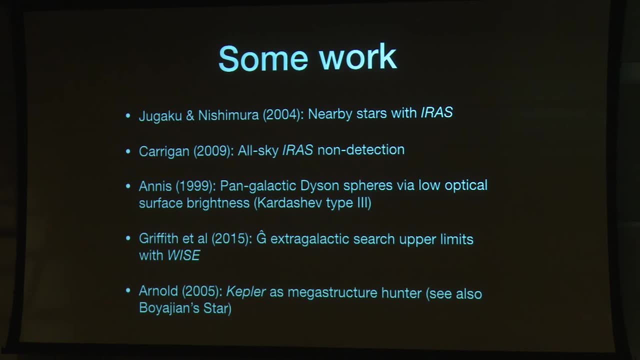 filamentary structures, And so that complicates the search for Dyson spheres even more. There's been a couple of studies, A couple of papers that have tried to look for this infrared excess, And so if you're interested in that work again, this will be provided to you later. 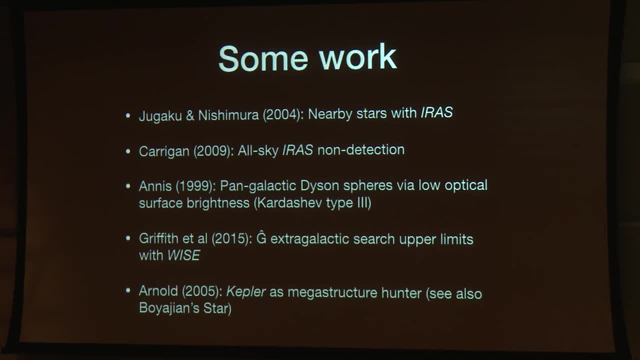 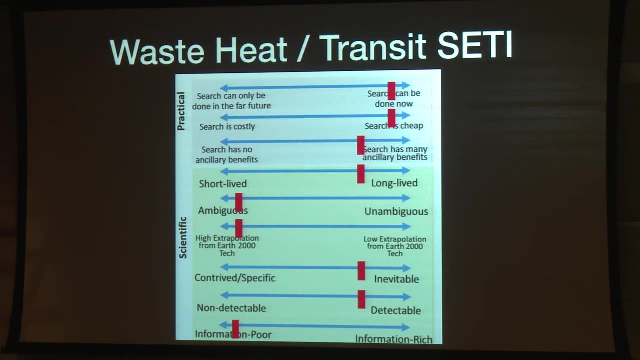 But in general this has been done with IRAS and WISE searching for these infrared excesses, And a lot of these papers have to deal with this problem of finding just very dusty objects, in addition to any candidates that they would actually want. So waste heat or artifact or transit. 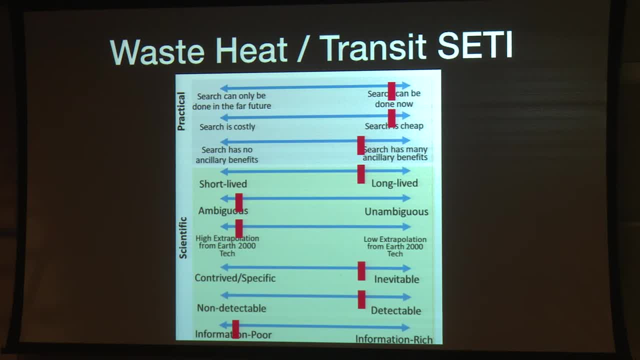 Or transit. SETI is sort of polarizing on the axes, as you can see, Practically, it's a great way to go about things because the search can be done. now You can perform this search on archival data, which makes it very cheap. 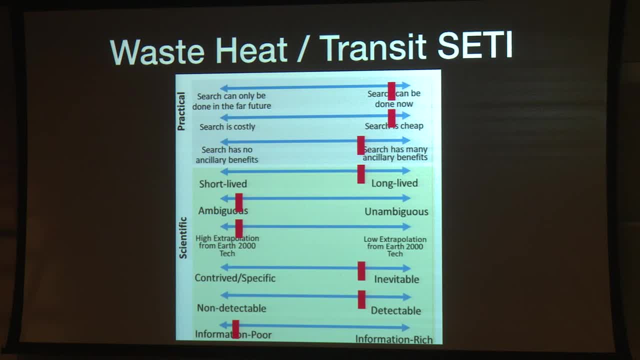 And if you don't find any, for example Dyson spheres, you've still found a lot of strangely dusty objects which are astrophysically interesting, And so, because you're looking for these anomalies, I've been using the Dyson spheres. 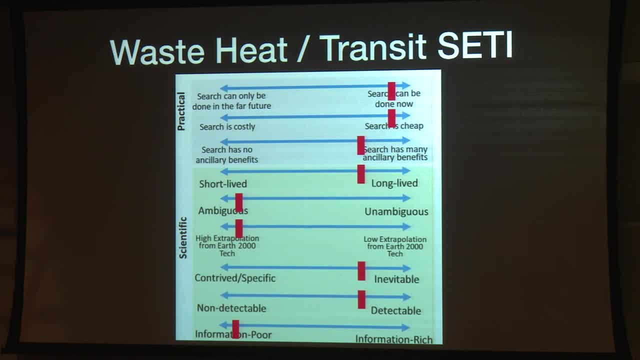 I've been using the Dyson sphere case, but you can apply this to almost any artifact. You're going to find interesting astrophysics, And so that's a very promising reason to pursue artifact SETI. At the same time, your signal is going to be longer lived than if you just assume a. 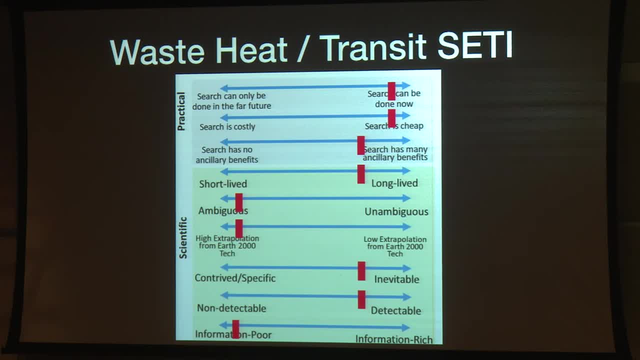 transmitter And using kind of the thermodynamics entropy argument, it will be inevitable, assuming that the building of a Dyson sphere is inevitable. But that's another question entirely And it is relatively detectable. You're looking for these large constructions. 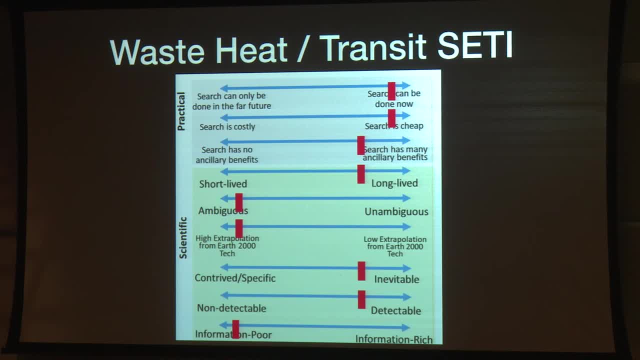 You're looking for things that have been built that we could detect And so kind of by construction they're going to be very detectable. Unfortunately, you have this ambiguity For Dyson spheres, you have the infrared excess problem And you have to assume technology that we have no way of. 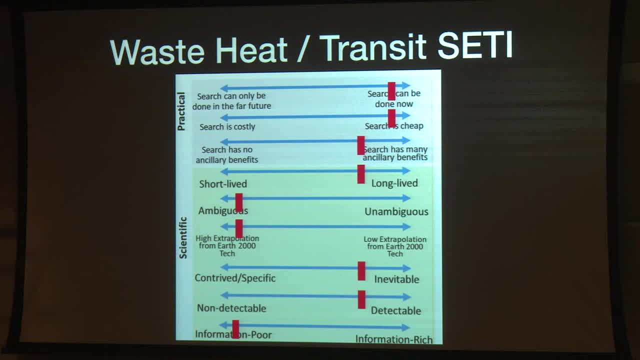 That we have no examples for on Earth. So you can't build a Dyson sphere with Earth 2000-level technology. So we have to assume that some development. So you can't build a Dyson sphere with Earth 2000-level technology. 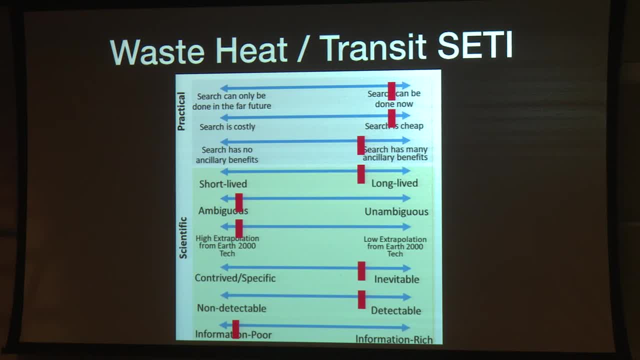 So we have to assume that some development. So you can't build a Dyson sphere with Earth 2000-level technology. So you can't build a Dyson sphere with Earth 2000-level technology. So we have to assume that some development happens that we are not sure of yet we have. 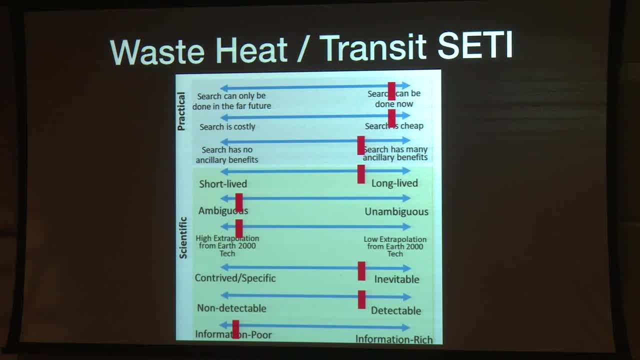 no example of in order to have these artifacts be built. And finally, the discovery of a Dyson sphere, for example, would be interesting, but it wouldn't necessarily tell us that much about who built it, why they built it, what they. 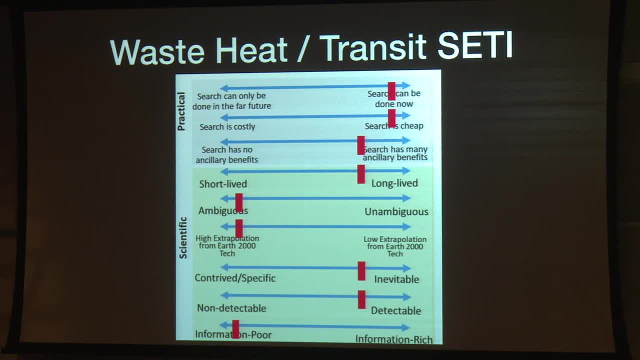 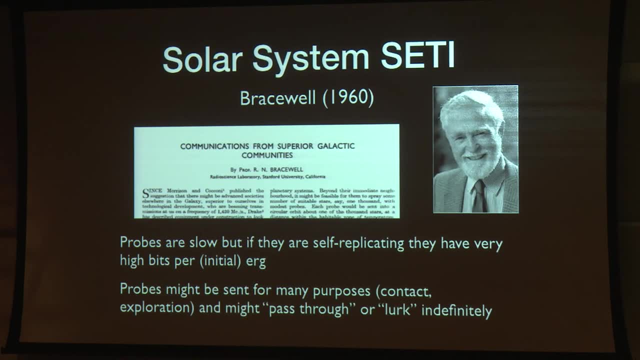 can do those sorts of things. You would just know that one was there. So on the same branch of artifact SETI, I'm going to move to solar system SETI. So instead of looking for artifacts around other stars, looking for artifacts around 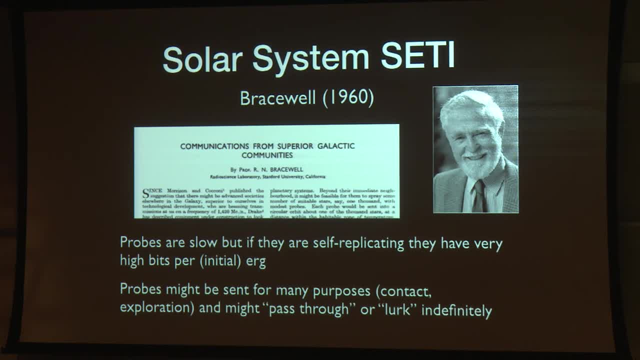 our own And again. Bracewell, in 1960, wrote this paper called Communications from Superior Galactic Communities and pointed out that sending probes seems like maybe not the best way to go, initially because they're slow. you have to wait for them to travel all the 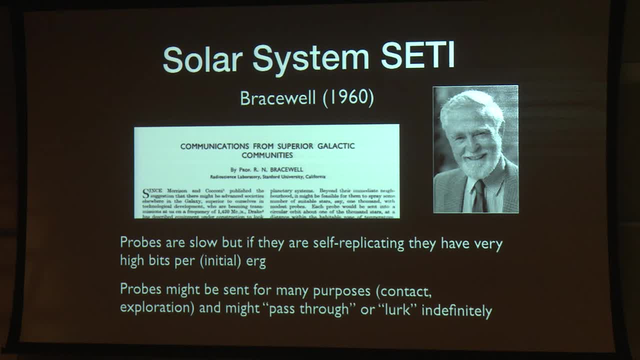 way to the next stellar system. But if you assume that that probe has something on it where it can collect resources and then duplicate itself, Then you get this exponential growth and maybe probes would be a good way to send a lot of information at a low initial energy cost, so long as you don't care too much about. how long they take to get there, And you might send probes for contact purposes, as in a lot of sci-fi, or you might just send them for exploration. They might pass right through stellar systems or they might lurk there indefinitely. So this idea used to be a lot more popular than it is now. 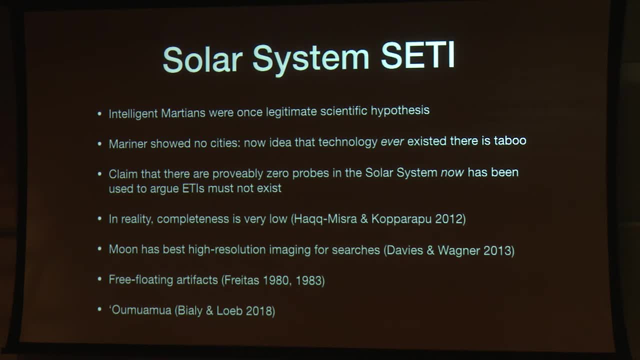 Especially when you have a lot of information, Especially when the exploration of Mars was a big thing in our space program And then Mariner showed that there were no cities on Mars and this kind of idea that had taken hold of the collective imagination went from really exciting to really taboo. 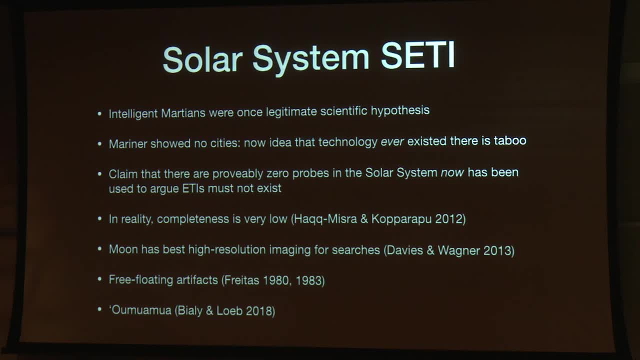 in scientific circles, And one claim that people use to say there is no extraterrestrial intelligence is the fact that we haven't found any probes in our own solar system. However, the completeness of our search within the solar system is not the only thing that 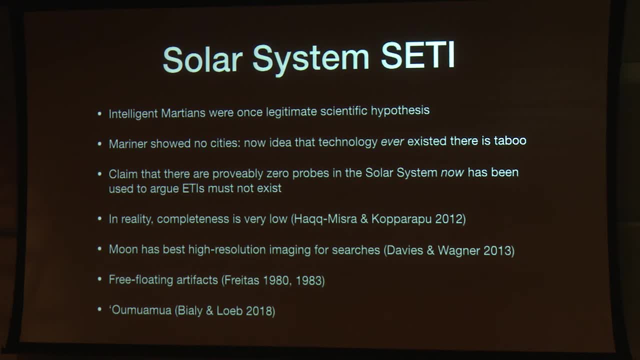 we haven't found any probes in our own solar system. It's the fact that our search within the solar system is actually very low And out of the parts of the solar system that we have imaged. if we're going to start somewhere, 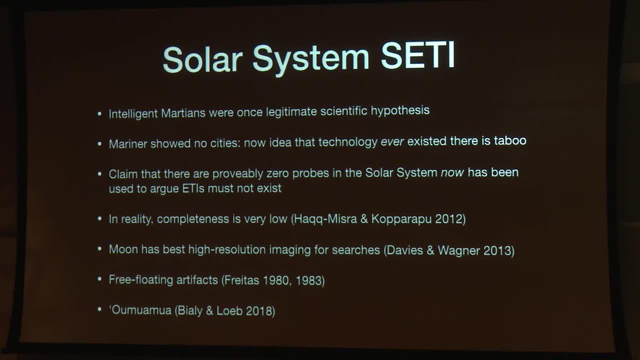 the moon is probably the best place to do so, But you could imagine looking on the surfaces of other bodies in the solar system. you could imagine looking in stable orbits, and you could even imagine looking at things that are just interlopers and pass through our solar system and leave, such as the recently. 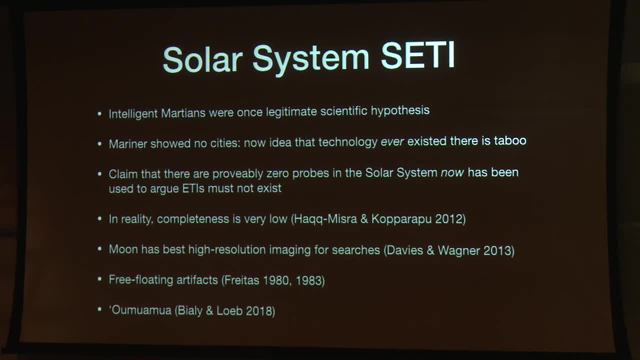 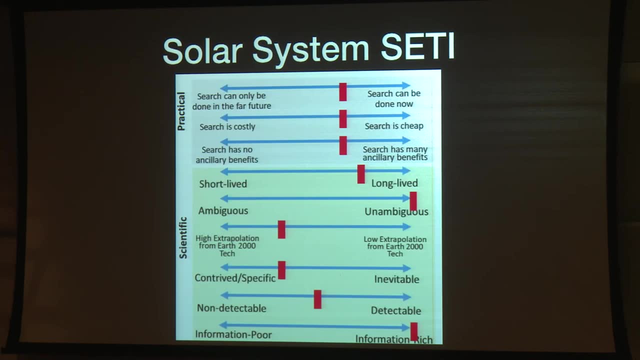 discovered Oumuamua And other Oh Extra solar system objects. So solar system SETI, again measured on these same axes, has a lot of benefits. Exploring our solar system is something that we do and can do now. 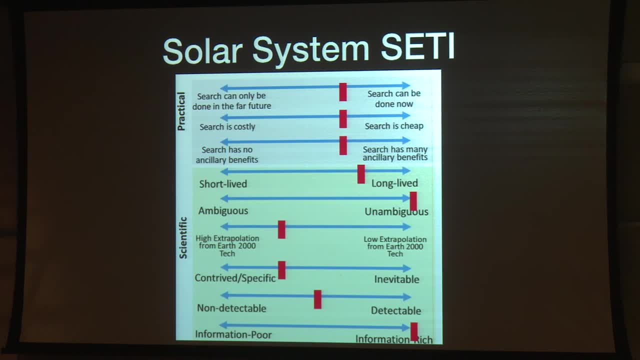 The search is cheaper depending on how well you integrate it with missions that already exist. And of course we want to explore the solar system, and so you can kind of integrate that with searches for biosignatures and other Satellites and rovers that we're already sending. 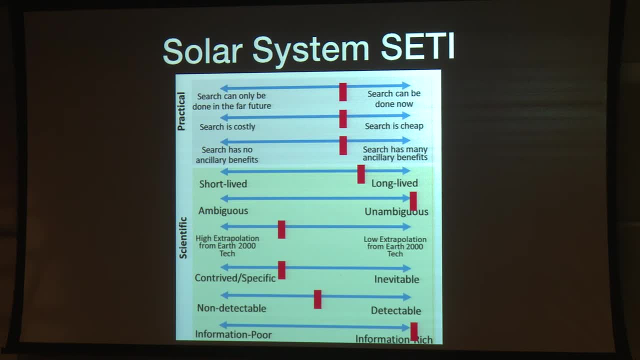 It has the benefit of: if we found anything, we would be able to examine it at close range and in situ, which we don't get with any other kind of technosignature. So it could be very unambiguous and information rich. 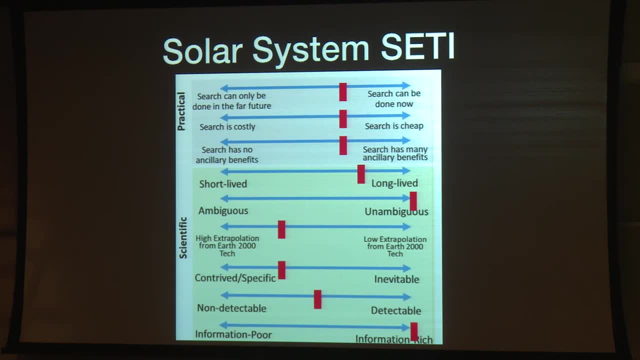 But it is sort of contrived. You have to assume that a probe was sent here And that would maybe require some extrapolation, especially if you're assuming the self-replicating probe idea. That's technology that we don't quite have yet. 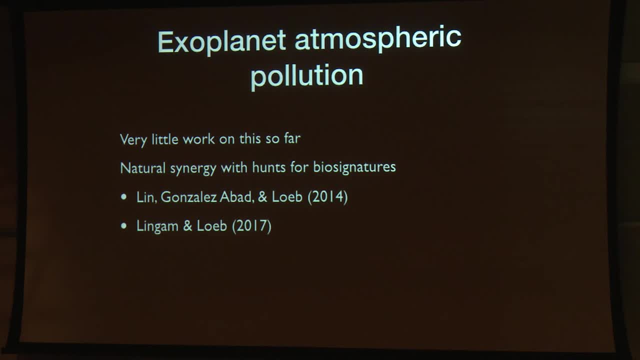 I want to briefly mention exoplanet atmospheric pollution, which is a very new area of technosignature searches, So there haven't been many papers too far on this subject. But looking for pollution in exoplanet atmospheres is promising because it synergizes really. 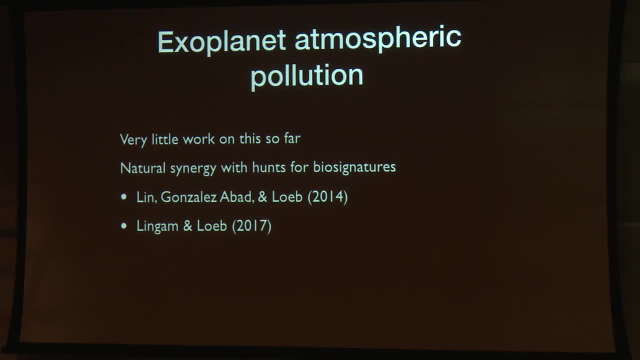 well with searches we're already planning to do for biosignatures in exoplanet atmospheres. So if we're already trying to take these high-resolution spectra, we might as well look for signatures of, say, chlorofluorocarbons in atmospheres or things like that. 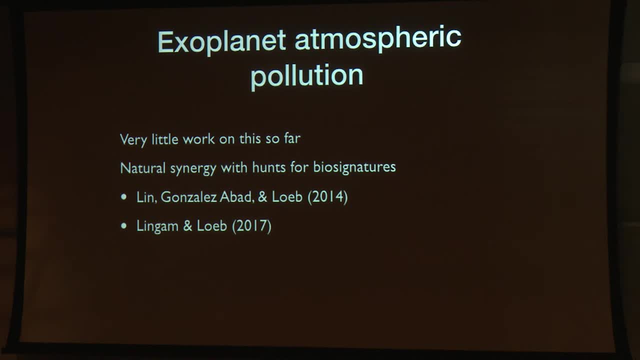 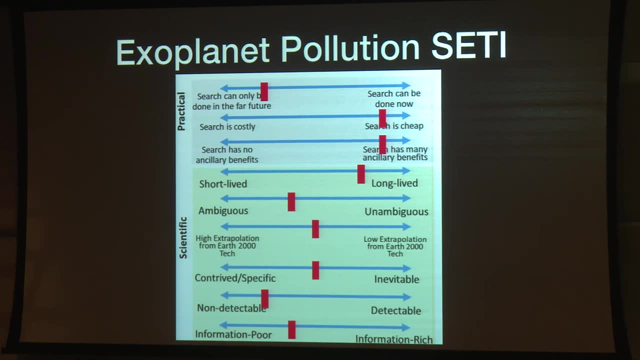 And so here are some papers that discuss this. And again, jumping back to these axes, unfortunately we don't have the instrumentation we need to take these high-resolution spectra. yet We're getting there- And that's something that is really in development- for biosignature searches. 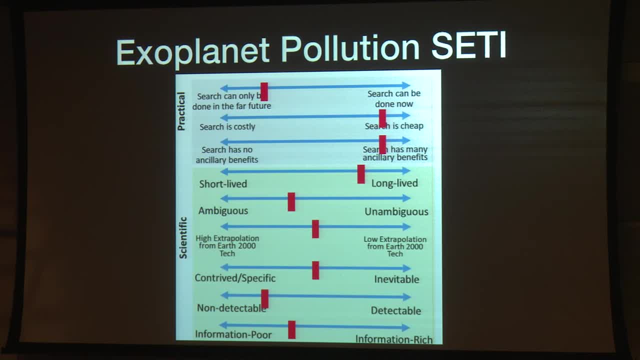 But it cannot be done right now. But once it can be done- because the search is going to be done anyway- it'll be cheap and have a lot of ancillary benefits to just kind of piggyback on existing biosignature searches. 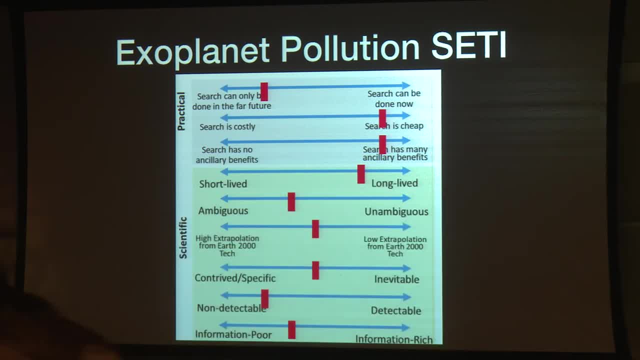 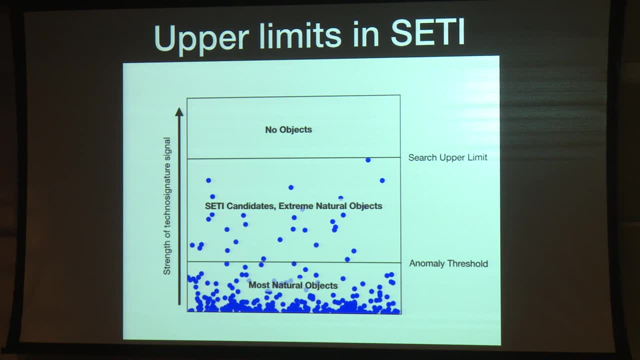 And the trick with these is mostly that they're going to be very difficult to detect, So it's more of a technology problem. So now I kind of wanted to lead up to some of the later talks that are going to be happening today. Why do we need anomaly detection? 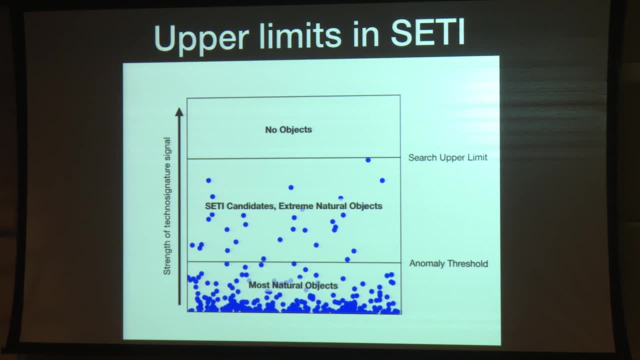 Why is that? something that's interesting to us in SETI, And I hope this kind of gives a little bit of a visual idea, which is that, no matter what you're talking about, whether it's asteroids, stars, galaxies, most of your natural objects 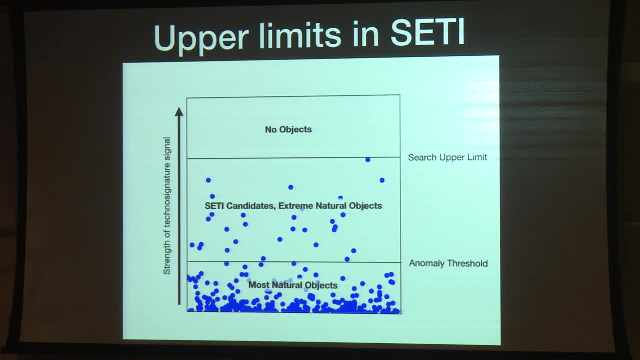 are going to have a set of parameters that's normal for that object And then, past some threshold, you're going to get objects that are a little weirder. You're going to get asteroids that are unusually reflective, or stars that have strange spectra, or galaxies that are unusually dark. 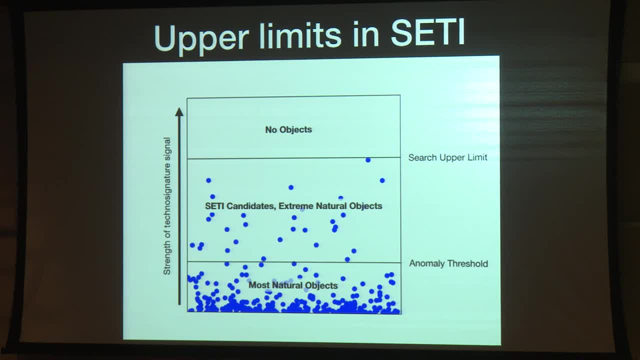 Right, Right, really red. And once you define that cutoff, that set of objects that falls above your normal parameters are going to be interesting and they're also going to be the ones that are most likely to be SETI candidates. And then there's some upper limit to your search. 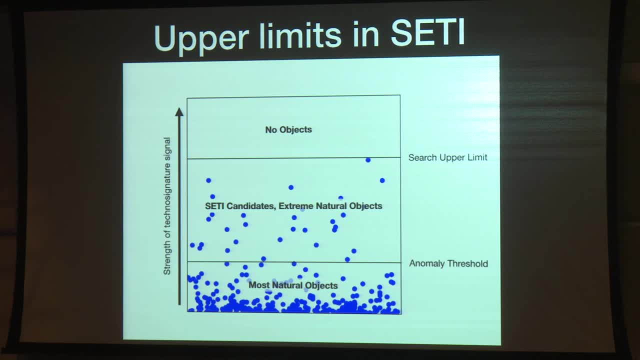 past, which there just aren't any objects anymore, And so that middle box there is what we really want to focus on, because that's a great way to take large data sets, take only the interesting things and then perform more detailed analyses of those objects. 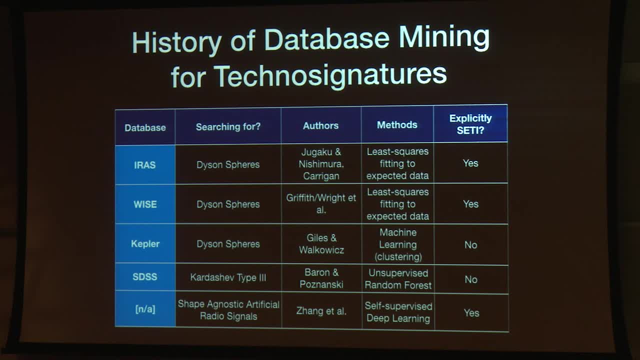 And historically. this is a slide that I just threw together and it is in no way complete, but here are some examples of the searches that have been done in this style, And most of these- actually, I didn't put years, but most of these are in the past 20 years, So 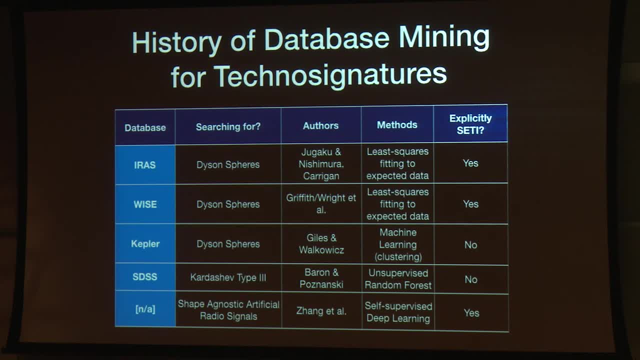 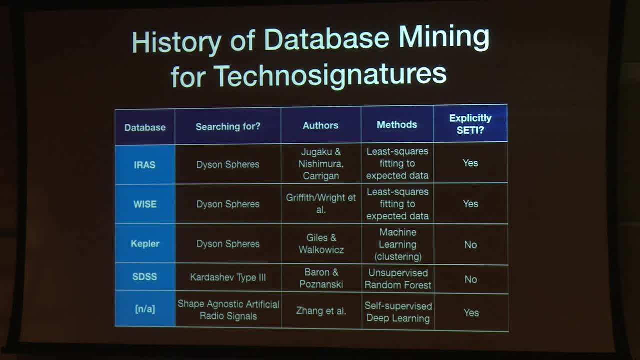 at the methods, only a couple of recent searches have actually used machine learning and other kind of newer techniques in data science to perform these searches, And so this is a really rich area that hasn't been explored that much yet, And hopefully I think it's something. 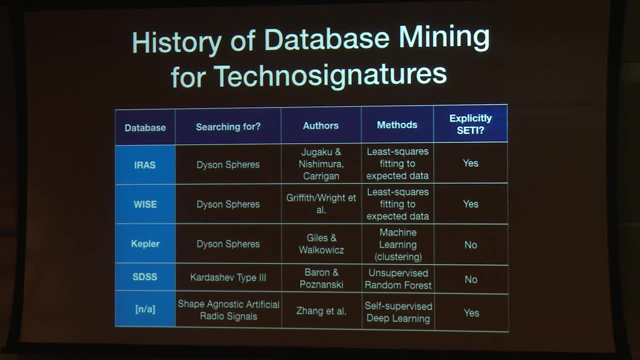 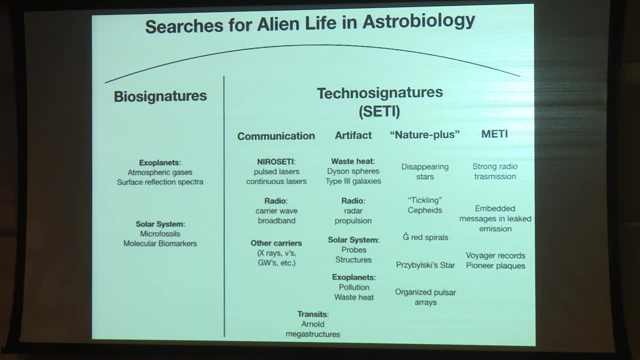 that we're going to tackle in this workshop. So with that, I'm going to leave this figure up if anyone has questions. But that's all I have And I'll take questions now, Thank you. 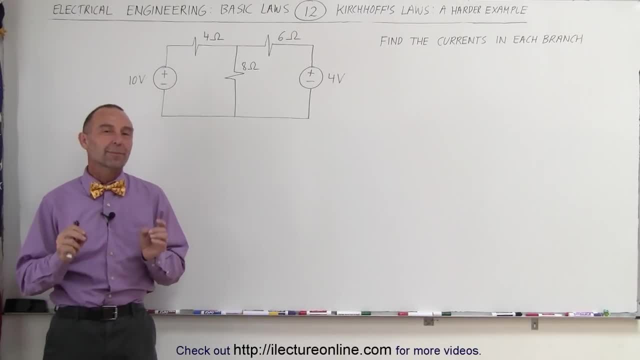 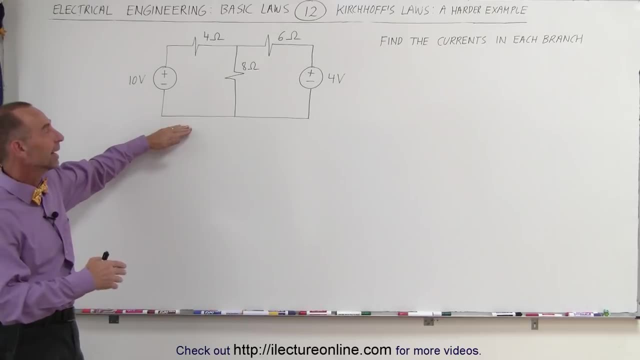 Welcome to Electro-Online Now. in this video, we have a more typical example of how to use Kirchhoff's rules. Matter of fact, in this type of circuit, Kirchhoff's rules is ideal, and the reason for that is we have multiple loops and we have multiple voltage sources. 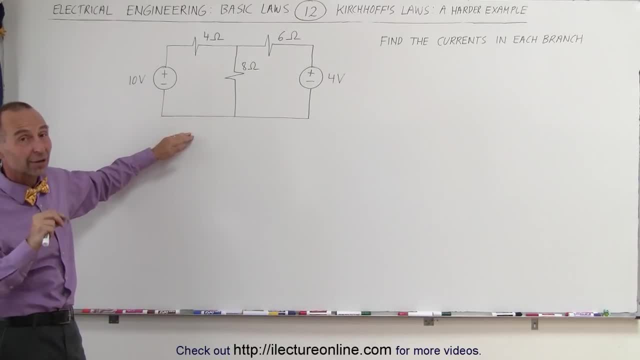 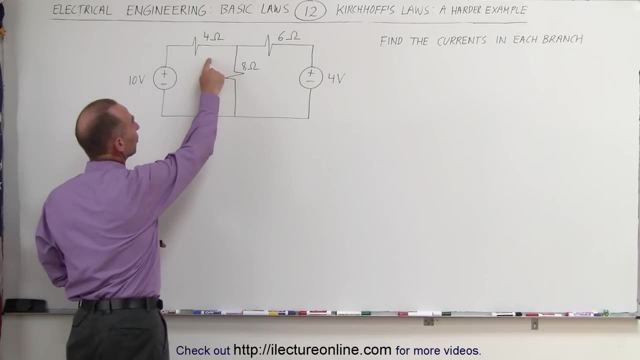 That's usually a good indication that you want to use- at least try- Kirchhoff's rules on this type of problem. We're supposed to find the currents in each of the branches. We want to find the current through the 4 ohm resistor, through the 6 ohm resistor and through the 8 ohm. 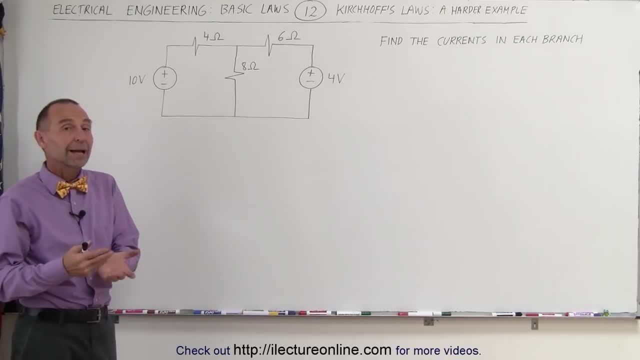 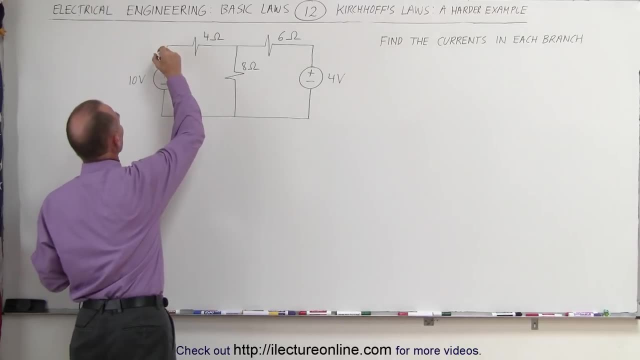 resistor. How do we do that? Well, we start out by assuming a direction in each of the branches. Since the positive end of the battery is on this side, I'm going to assume that the current flows in this direction through this branch, and I'll call this I1.. Here we have the voltage source. 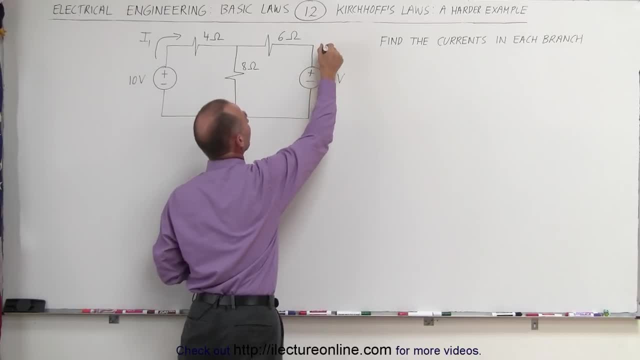 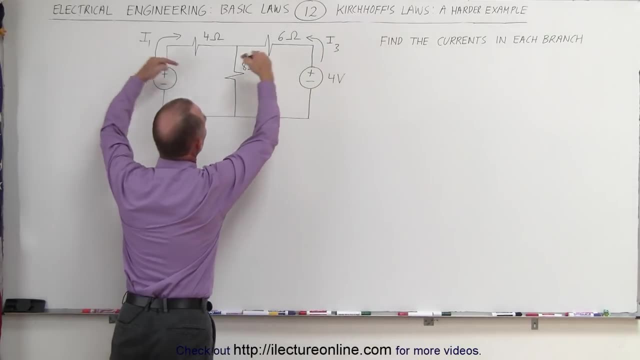 with the positive end on this direction and on this side. so I'm going to assume that the current flows in this direction, through this branch, so let's call that I3. Then, through this branch, if the two currents come together, we can assume that the current 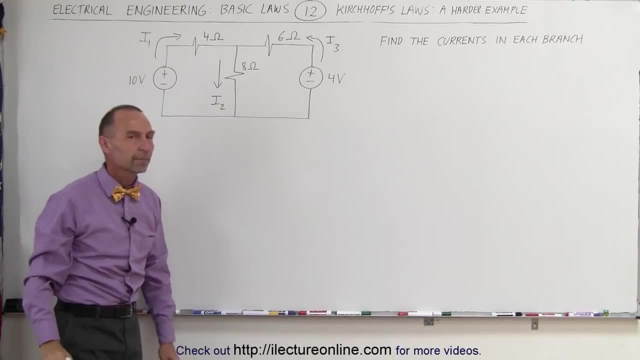 will flow in this direction through here. let's call that I2.. Now, I may be wrong. it could be that I3 is actually in the opposite direction, that the voltage, the potential difference across this battery is so large that it overwhelms this one and sends current in this direction, that 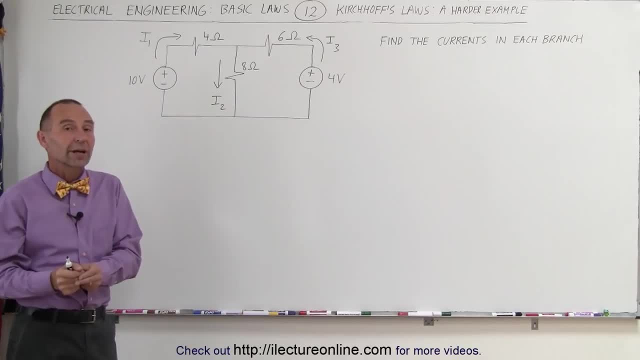 is possible. It doesn't matter if we assume the wrong direction. in the end, if we assume the wrong direction for I3, the answer will come out negative, which then indicates it's actually in the opposite direction direction. so you don't have to sit there and worry- oh, did I get that right? Even if you.